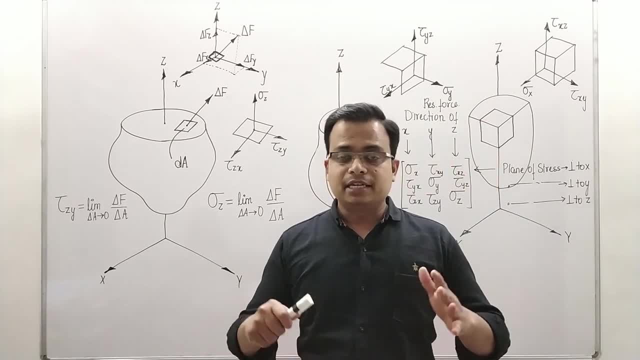 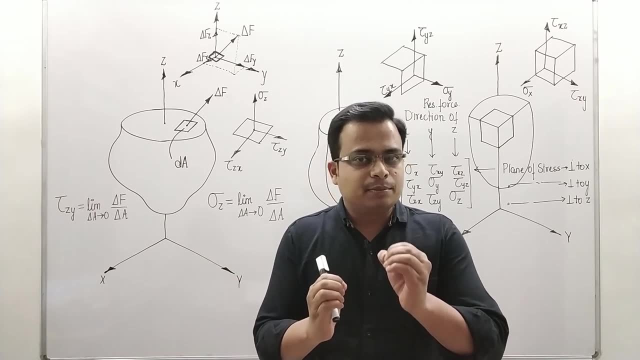 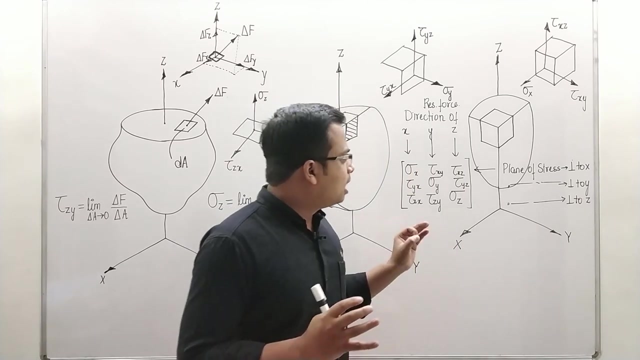 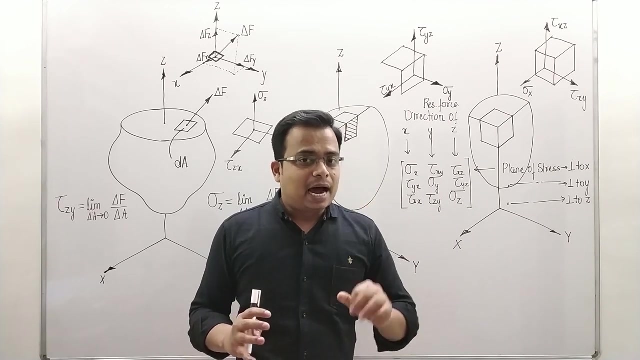 Hello everyone, this is Manas, your friend and tutor, And guys. I promised you that I'm going to be rolling out videos on principle stress and strain, But before that, you first need to understand how stress at a particular point inside a rigid body can be worked out, And you'll be amazed to hear this- that stress has as many as nine components, nine different components, out of which three are normal components and six are sheer stress components. And this is this is really, really amazing. 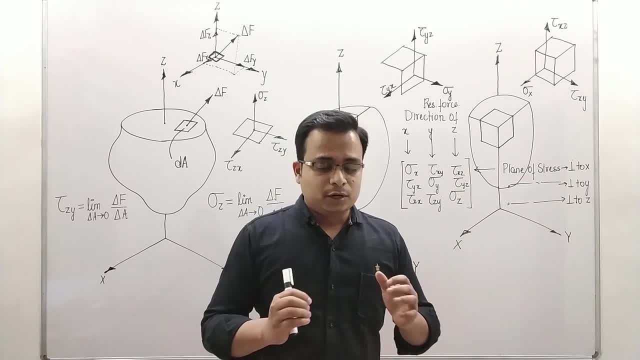 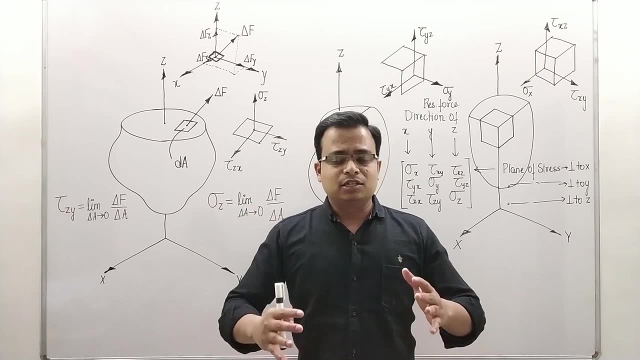 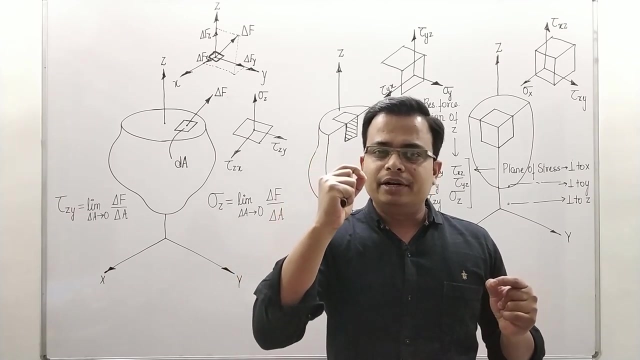 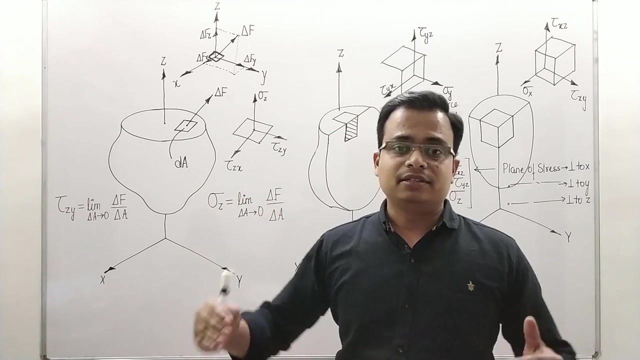 And this is something that we'll try to work out in today's session. So today, basically, we'll pick up a rigid body, we'll cut, we'll slice, we'll dice: Okay, this is, this is nothing less than a post mortem of a rigid body, And we'll try to work out the stress acting at a point inside that one. Today's session is going to be very, very interesting. There are a lot of diagrams. as I told you, cut, dice and slice. Here we go, Let's start. 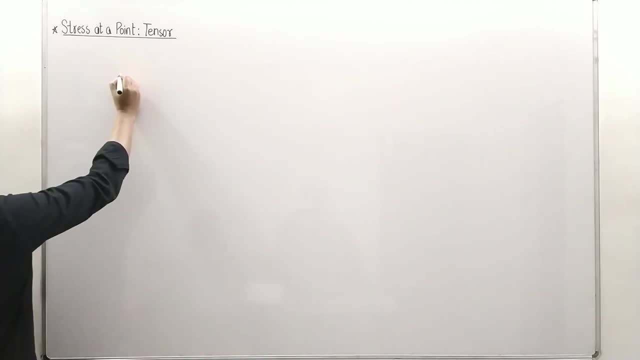 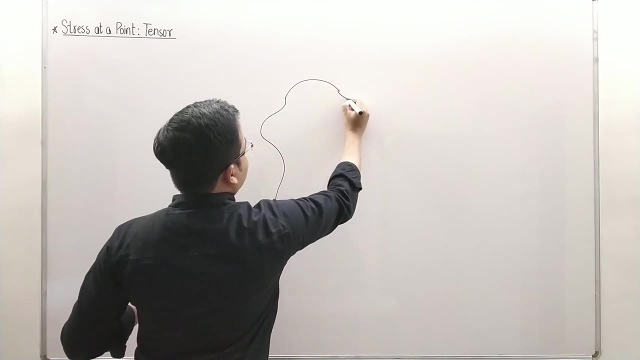 So let us start today's session by first making a rigid body. Let me draw it over here. So it's something like this. Let's say: like this, Okay, And like this: Right. And now a bunch of forces are acting on this rigid body. 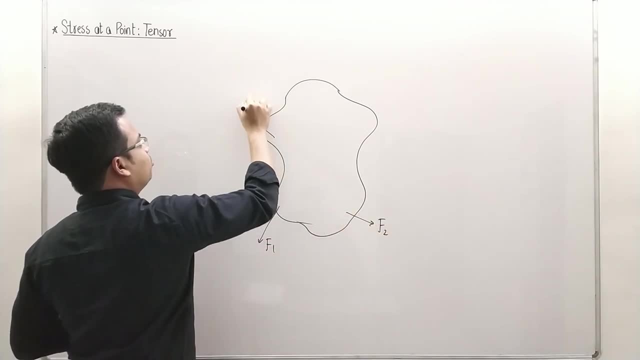 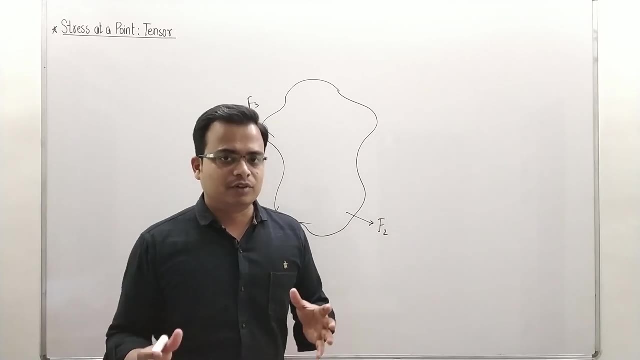 We'll first cut this. Okay, this is the uncut rigid body. let's say, a bunch of forces- F1, F2 and F3- are acting on this. So inside, you know very well that there is going to be some resistance offered. 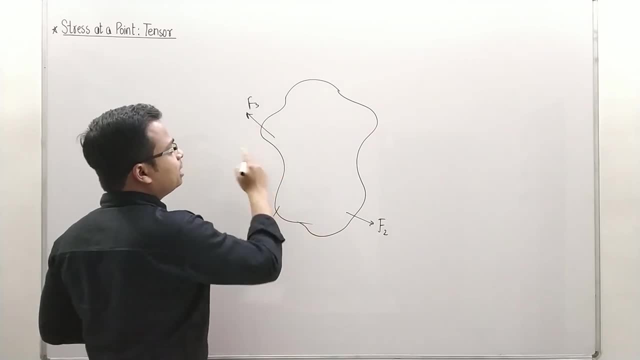 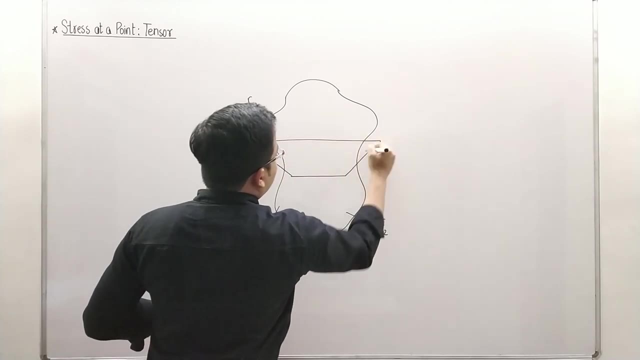 by the material, obviously. So there are going to be resisting forces which are which will set up inside this rigid body. So let me just cut this body by, say, a plane like this, a horizontal plane, And in that case we'll be considering a section. 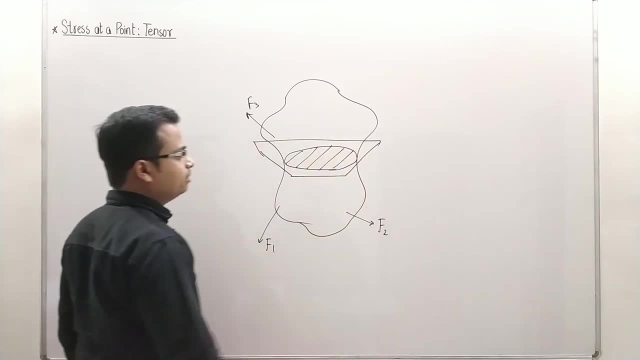 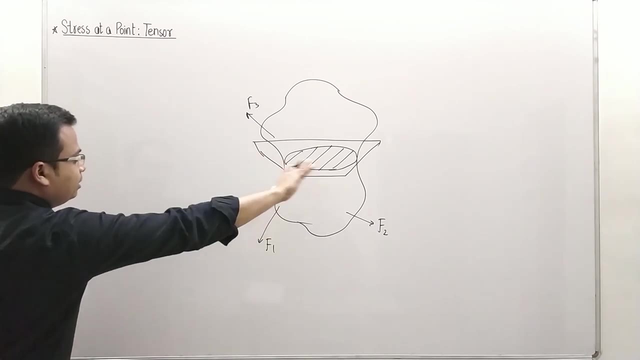 Okay, and we'll try to see what's happening inside this. Okay, how is the nature of forces on different points? So let me try to make a figure over here. Okay, the cut section with the help of horizontal plane. Here it is. 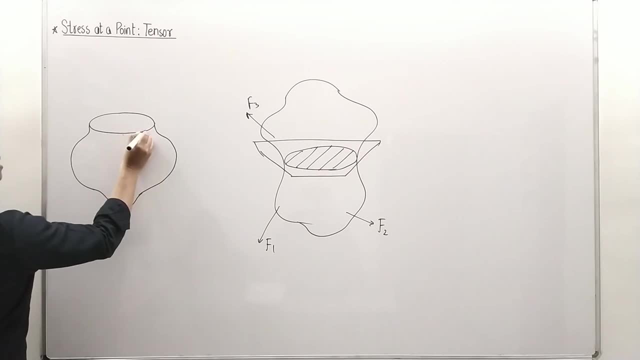 And we've got three axes, as usual, which will be perpendicular axes. this over here is the Z axis, then we've got a Y axis and an X axis right here And, by the way, they are perpendicular. X, Y and Z are perpendicular- three mutually perpendicular axes. 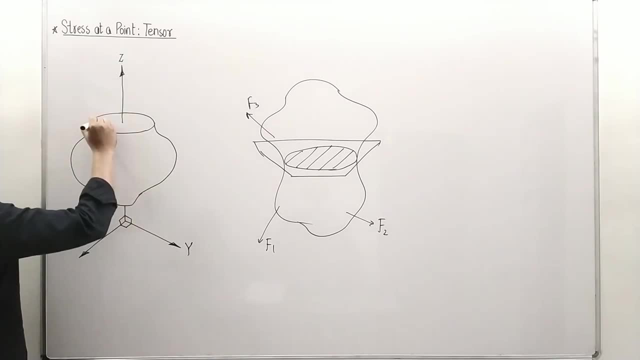 Now there will be resisting forces, isn't it? These are all resisting forces. I can make a bunch of resisting forces Right now. let me rub all of this. We'll try to focus on a particular area. What are we doing? We are trying to find the stress at a particular point. 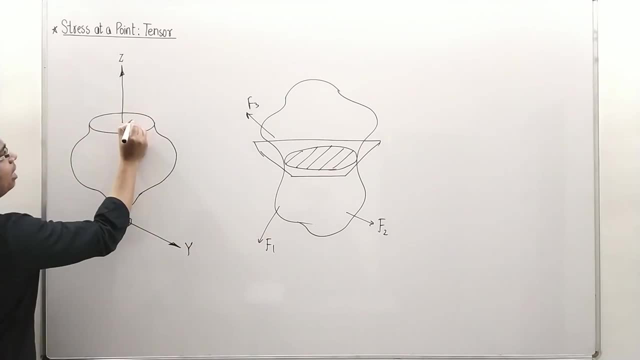 So first of all, let me consider an area and then let us try to analyze. Let's say, we are talking about this area Like this: okay, Yeah, pretty good, What is happening over here? There must be some force acting. 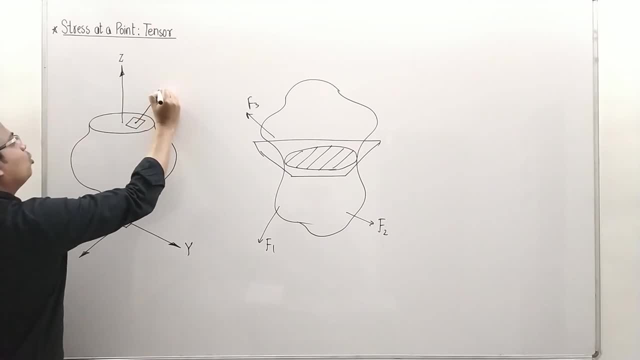 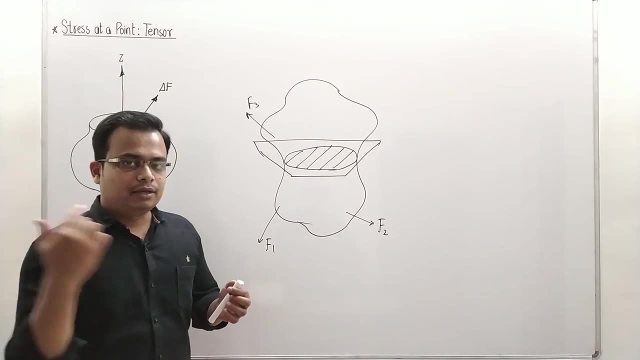 A resisting force acting like this. Let's call this force by delta F. Now this force is in space, So obviously this force is going to have components in the X, Y and Z directions. So let us try to make that. And first of all let me rub this: 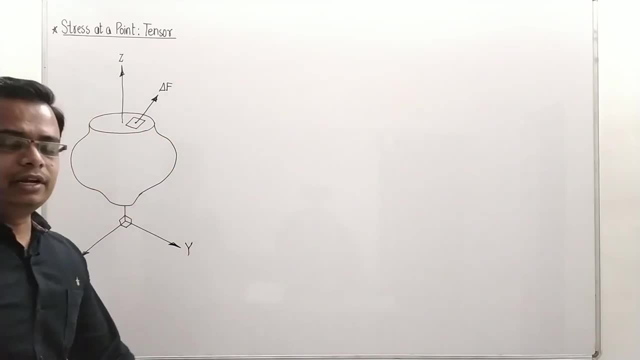 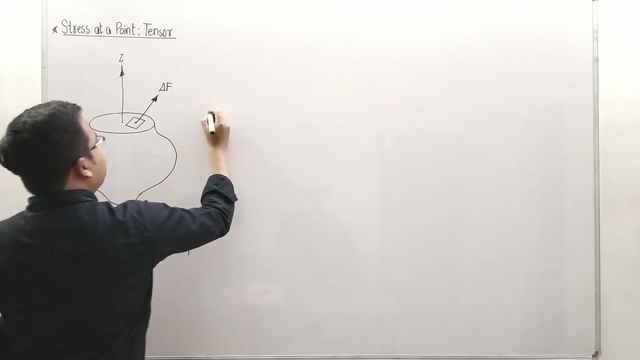 Okay, then we'll try to analyze everything. you'll get to know what normal stress is. you will get to know what shear stress is by definition. So here we go. So let me have the components of force. So first of all, let me make the axis. This right over here is the z axis, Z axis, This is the y axis And this right here is the x axis. So we've got a plane over here like this. Let me make this plane. 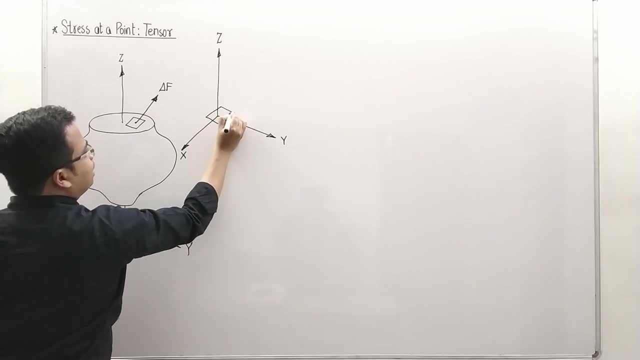 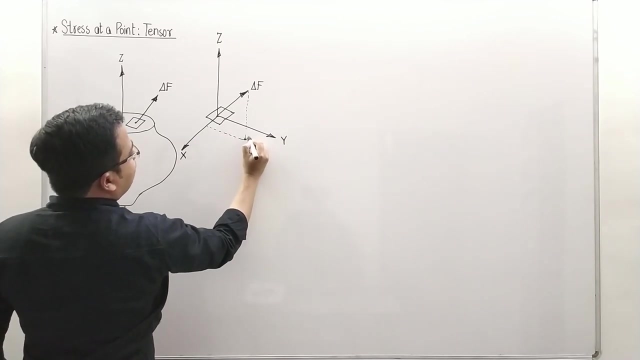 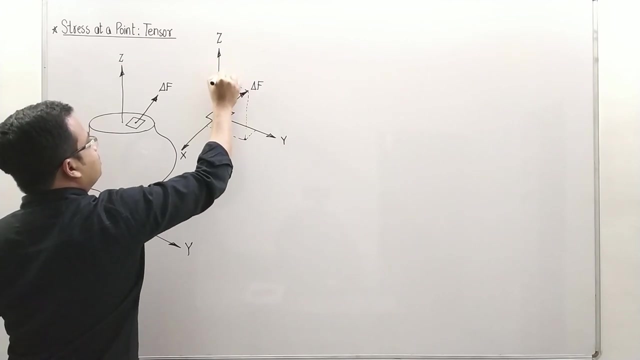 Okay, And on to this plane. this force is acting. The name of the force is delta F. Done Now, this is going to have components, So there is going to be an x component and there is going to be a y component And also a z component. This, by the way, is the z component: Delta F z. 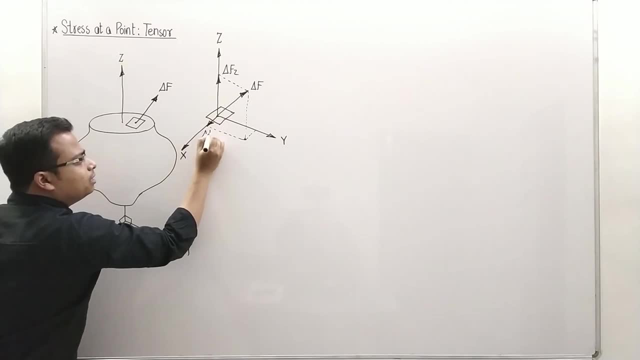 And this over here Is delta F. Which one is this? Delta F x? Now you've got to watch this video right till the end. If you have started, then do watch it right till the end, Because you'll get to know a lot of things, And you'll finally get to know why stress is a tensor And how the matrix is drawn. 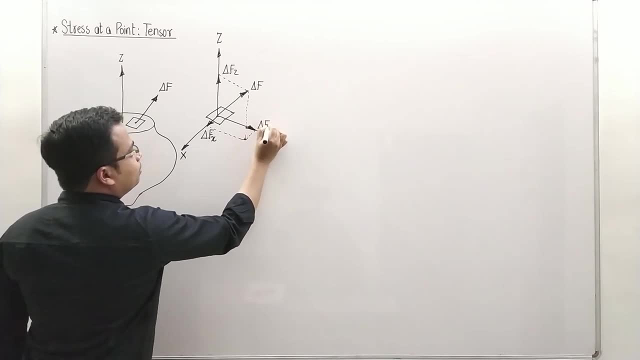 And this is delta F? y. Okay, Two things which I need to tell you. first of all, Force and area. You know that stress is defined by The resistance offered per unit area, Isn't it So? here, this is the area. 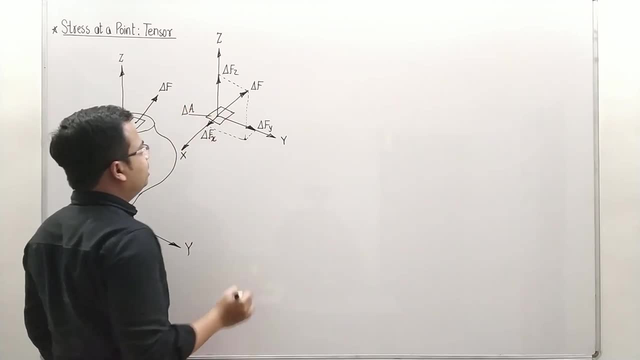 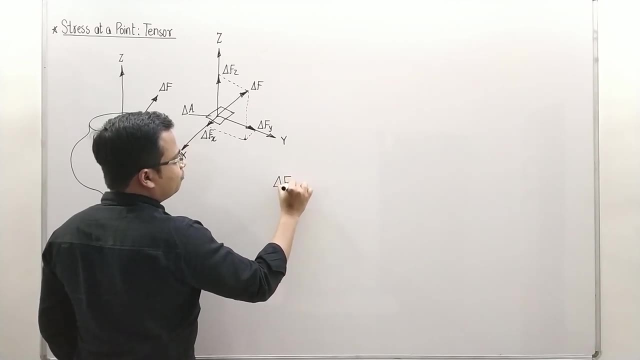 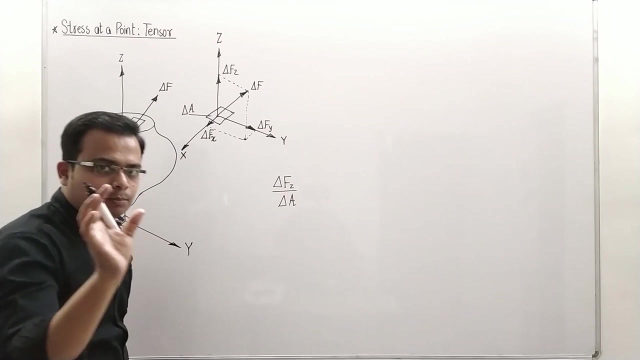 And let's say this is a very small area Written as delta A. So watch this. What about this Ratio? Delta F, let's say, z Over delta A. We want to find the stress at a particular point, At a point. 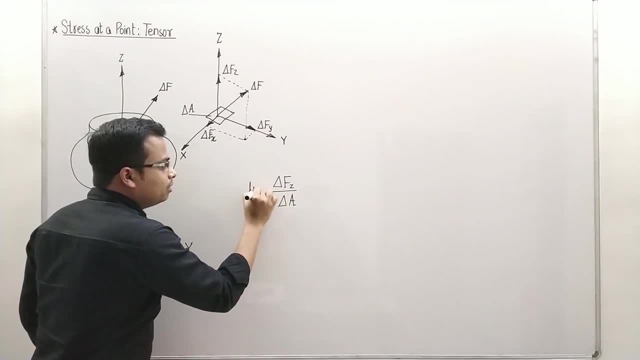 So the area has to be very small. The area has to be such That it has to tend to 0.. Area tends to 0. Then only we'll be able to find the stress at a particular point And, by the way, this is known as normal stress. 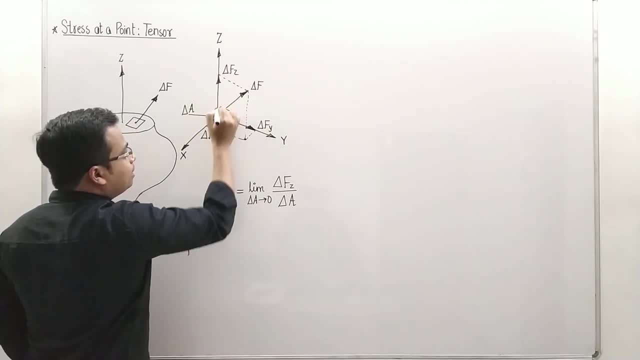 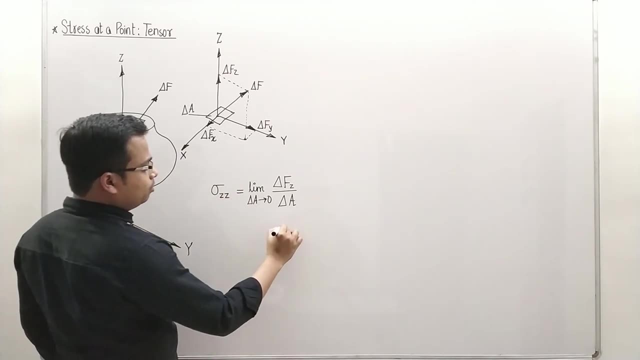 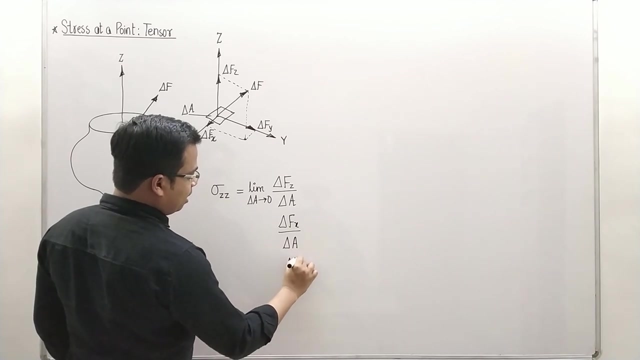 Why normal? Because this delta F- z is actually normal to this area, Isn't it? So this has been written as delta, not delta, but sigma z z. One more thing which I need to tell you is about this ratio: delta F x over delta A and delta F y over delta A. 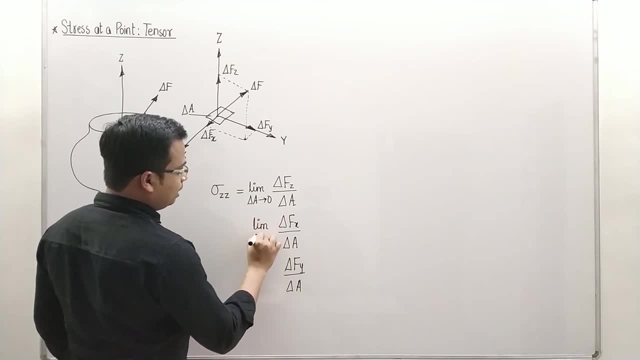 Now, both of them, or for both of them, area will tend to 0.. Why? Because we are trying to find the stress at a particular point. Area will tend to 0. And this, by the way, this, by the way, this, is nothing but the shear stress. 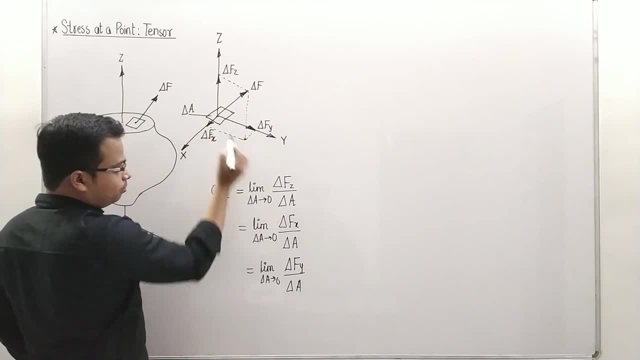 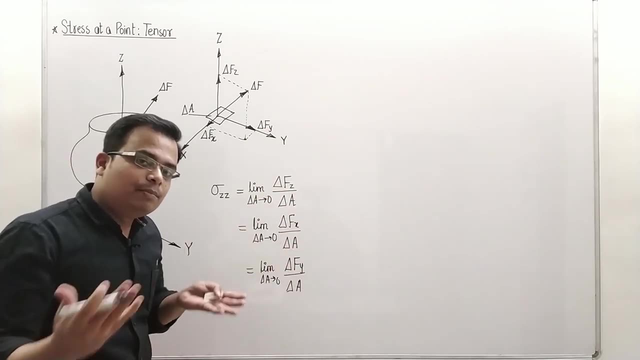 Why? Because this force, this force F? y, this is F? x, this is F? x and F? y. Both of them are along the plane or tangential to the plane, So the stress induced will be shear stress. So this has to be written as tau. 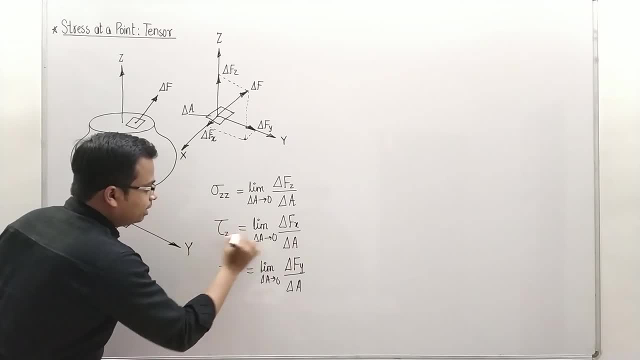 This also has to be written as tau, And I'm going to write over here: tau z, this is x in the direction of x and this is tau z in the direction of y. Now some of you guys might be thinking: what is this subscript notation all about? 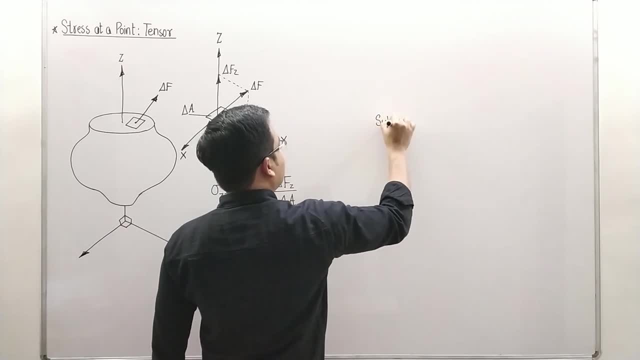 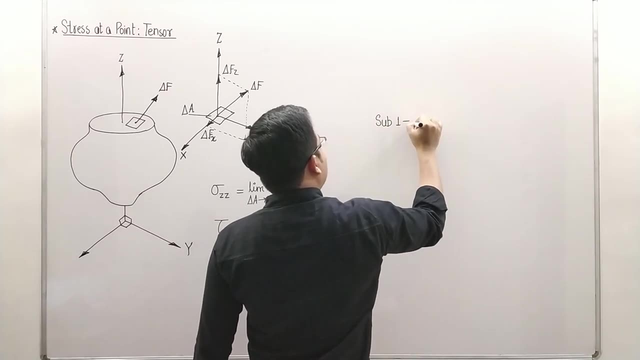 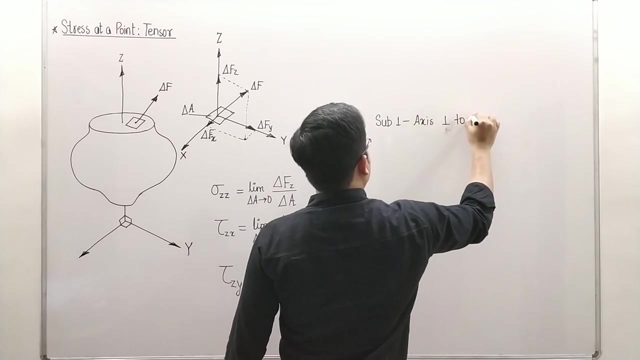 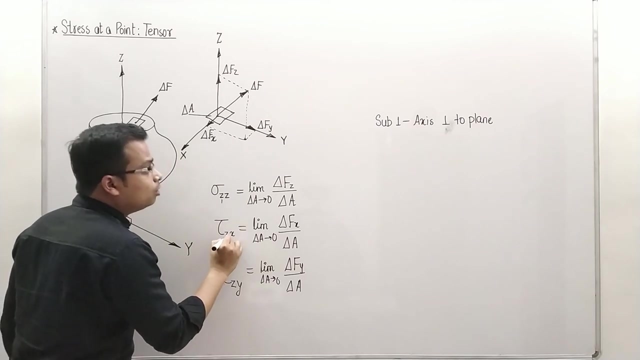 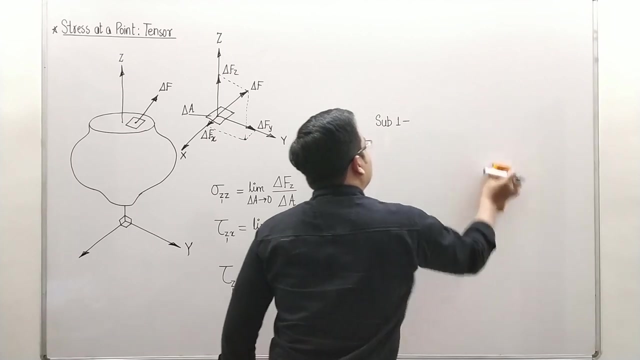 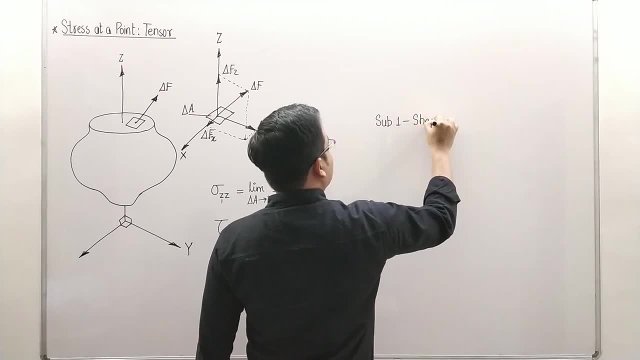 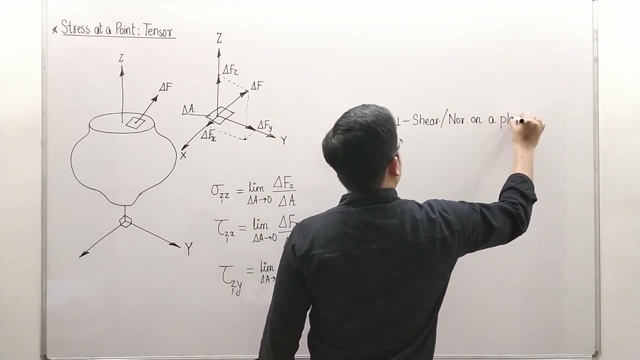 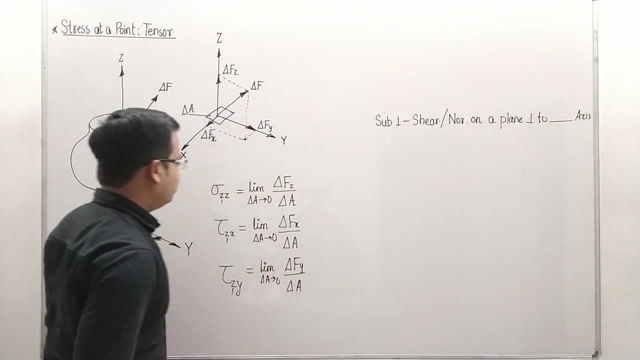 One refers to shear stress or normal stress on a plane perpendicular to dash axis. So if it is z, that means on a plane perpendicular to z axis. if it is x, then there would be plane perpendicular to x axis. What about subscript 2?? 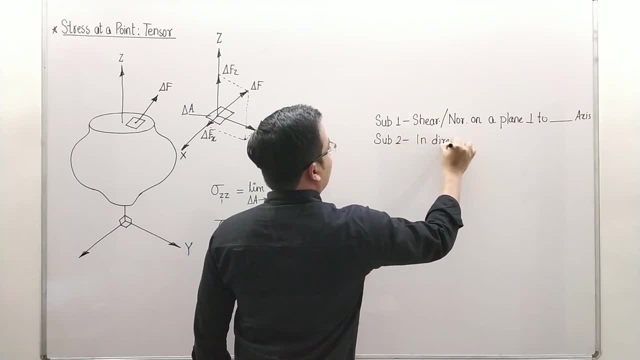 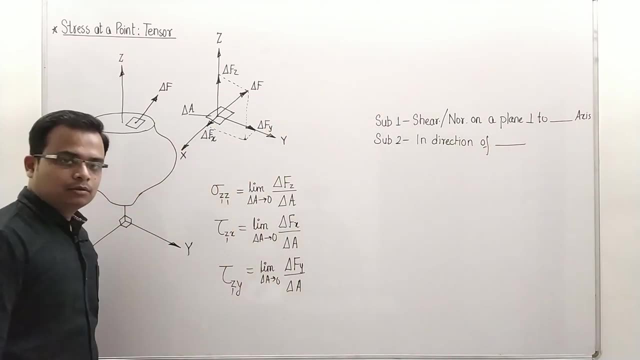 Subscript 2 is very simple: in direction of, In direction of what? So here it is subscript 2.. So let me recap Subscript 1 and subscript 2 together. Normal stress sigma is for normal stress, by the way. 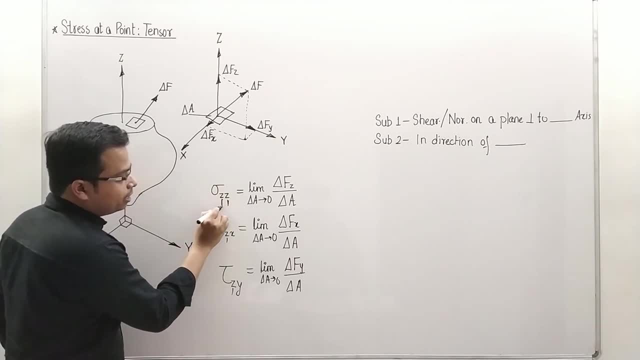 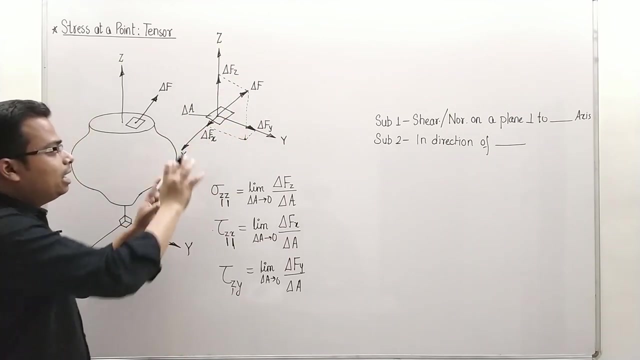 Normal stress on a plane perpendicular to z axis in the direction of z. Shear stress on a plane perpendicular to z axis in the direction of x. So this way: shear stress on the plane perpendicular to z axis in the direction of x. I will explain you all of that stuff once again. 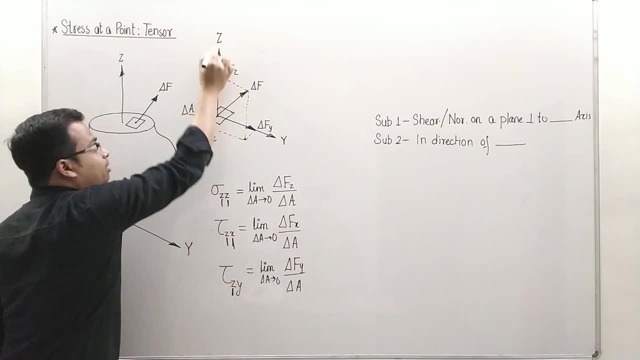 And this is finally shear stress on a plane perpendicular to z axis. Perpendicular to z axis. we have got this plane and there is this Shear stress will be acting along this direction. We will be making that also, Don't worry. 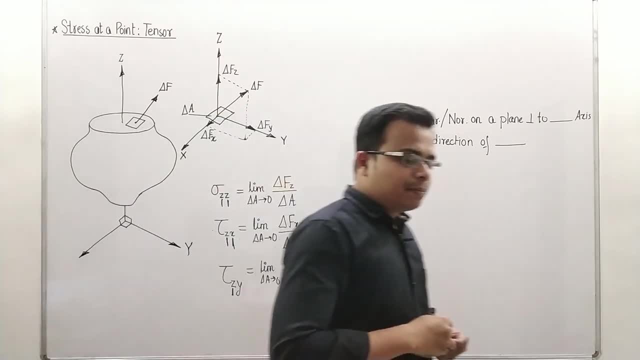 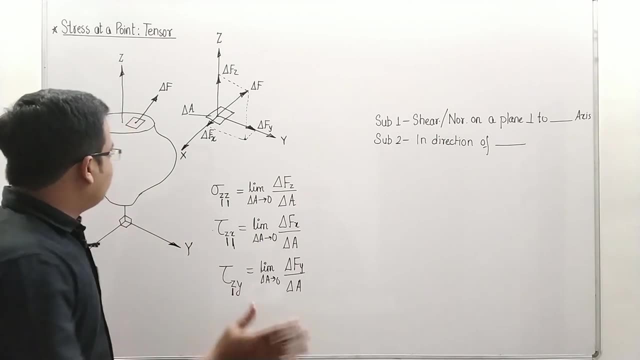 Okay, So this was all about basically how stress acts at a particular point. Now let us do one more cut section. And now let us do one more cut section. And now, Basically, what we will try to do is we will try to cut it with the help of a vertical. 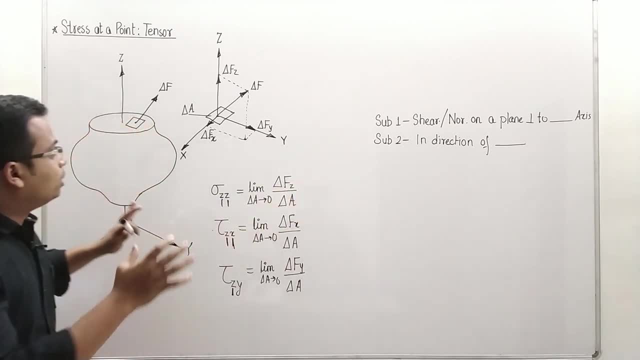 section Let us see what is in store. So, whatever I have written till now, you should note this down. because the board is a bit small, I need to rub, keep on rubbing this stuff, Okay, So, so, so, so where shall we move? 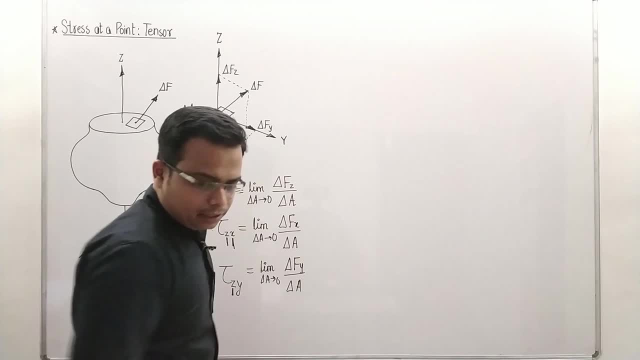 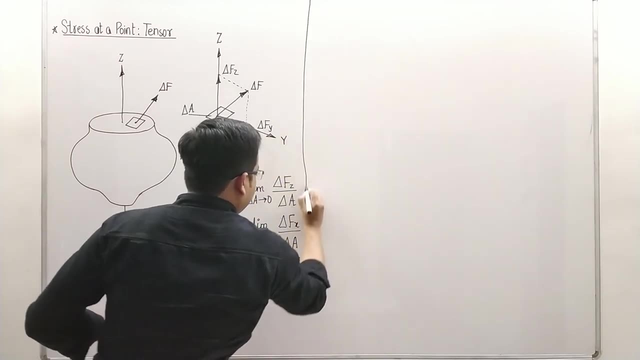 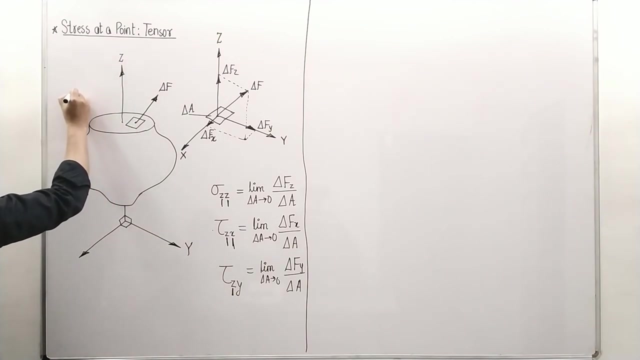 Okay, Okay, Let us now use this much space For the remaining two sections. Okay, Okay, One more thing. As far as this plane is concerned, let me make a bigger figure. not this way, but okay, So I will refer to this as the top plane. 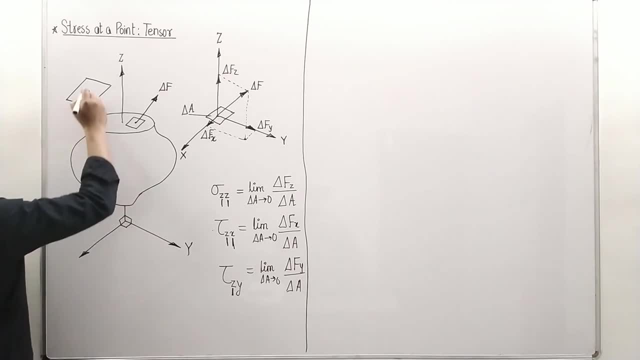 How many stresses are acting? So there are three stresses which are acting onto this plane. One is in the z direction, The other one is in the z direction. This is sigma z. So this can can be written simply as sigma z. 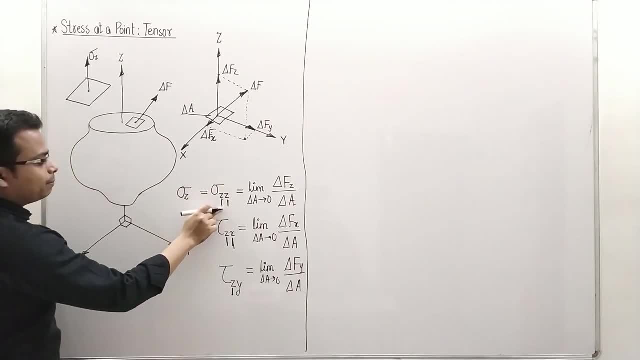 Okay, Okay, So perpendicular to z axis, on a plane, perpendicular to z axis, and also in the direction of z, in the direction of z, That is it In the direction of z, and also perpendicular to a plane, this plane which is perpendicular. 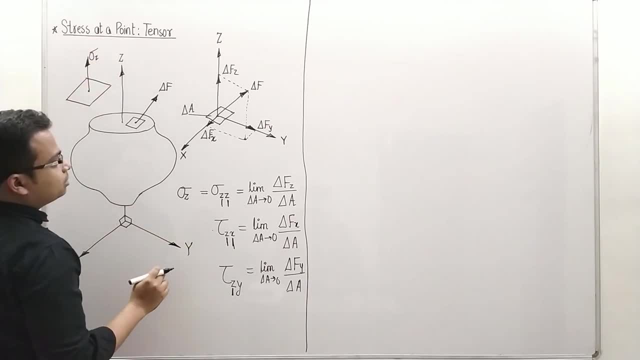 to the z axis, you can say. Then there are two more shear stresses: One is along this direction, One is along this direction, So let me just put it over here. So what the name is: tau, on a plane perpendicular to z axis, in the direction of in the direction. 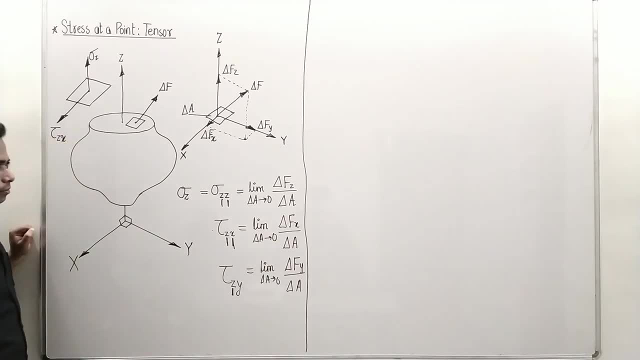 of x Done. There is one more shear stress acting here, and this is also on a plane perpendicular to the z axis. and in which direction? In the direction of y. So this has got to be written as tau z y. So there are three stresses. 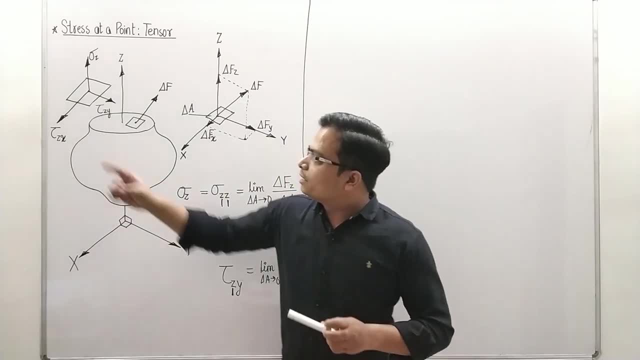 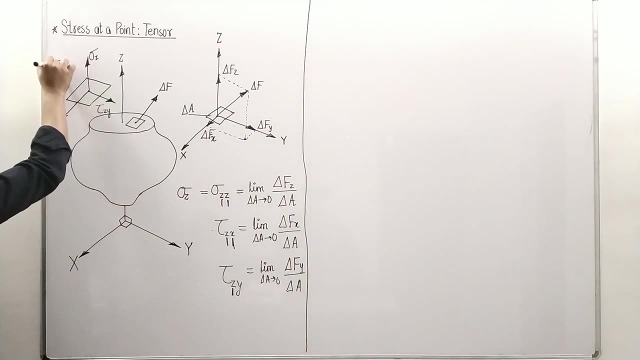 Okay, Okay. There are three components of stress acting on a particular plane, right? So this was all about the top plane. Let me just refer to this plane as the top plane. Now let us try to analyze what happens on a front plane and what happens on a side plane. 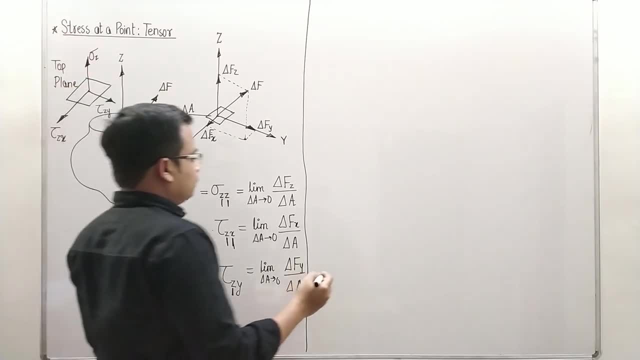 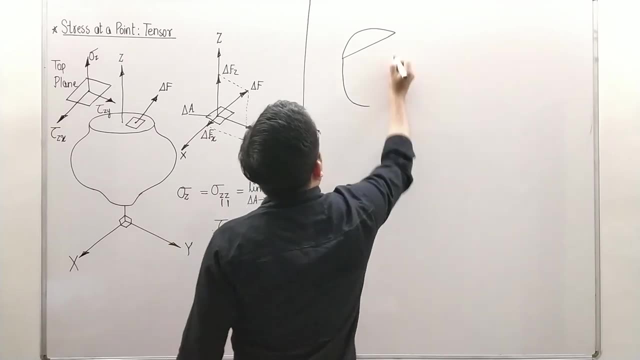 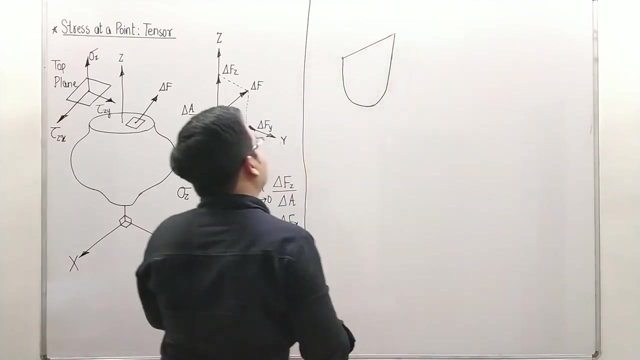 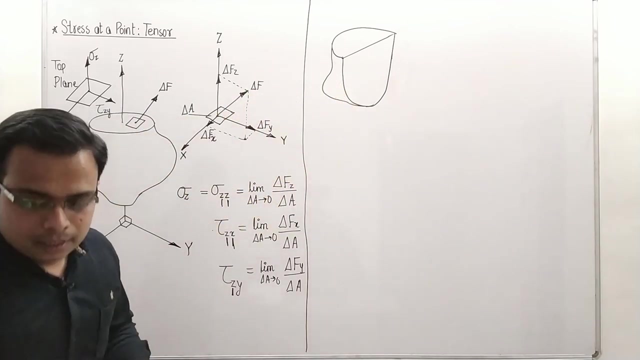 So I've got to cut this with the help of a vertical plane. Again a cut. Here we go. I've cut this with the help of a vertical plane. This looks nice, Okay, So we've cut it up. Now let me make the axis. 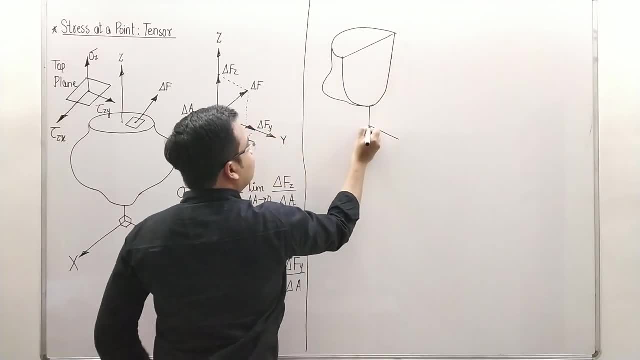 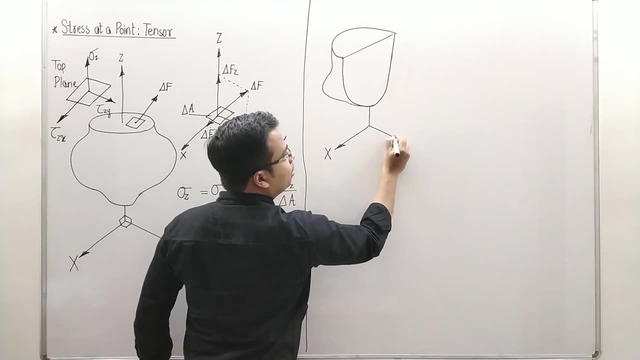 This, This Don't make it- And this. So this right over here. What was it? X, That's x, That's y, And we've got one more axis. So this right over here. What was it? X? 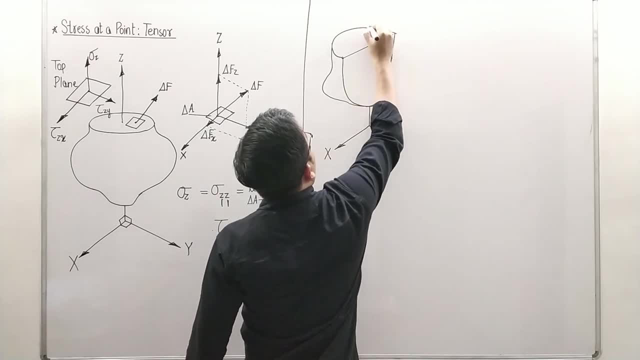 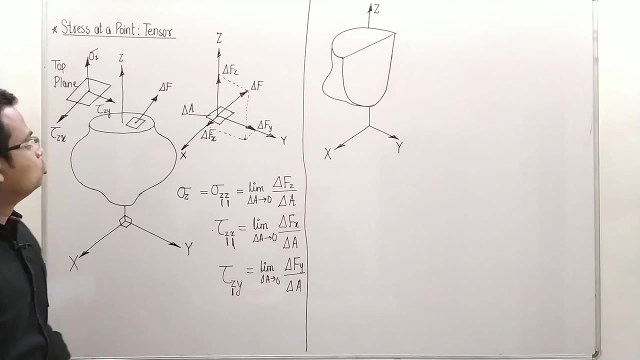 That's x, That's y And we've got one more axis Over here. This right here is the z axis, right. So we already know what is happening on the top plane. We already know what's happening in the top plane. 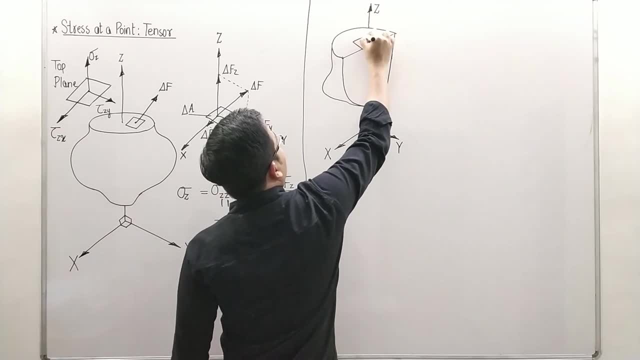 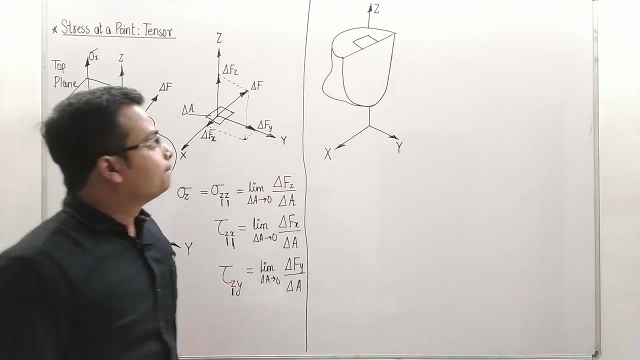 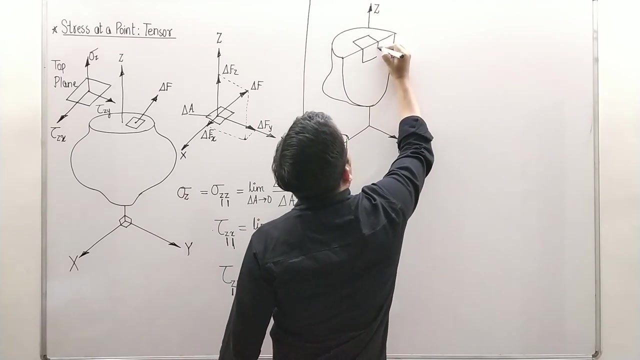 Let me make that top plane once again. So this right here is the top plane. You know what's happening over there. There are three components of stress: One normal and two shear. We want to know what's happening in this plane. So, as you can see, let me try to make this plane. 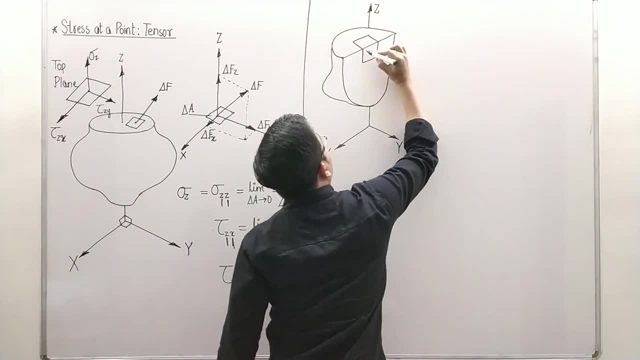 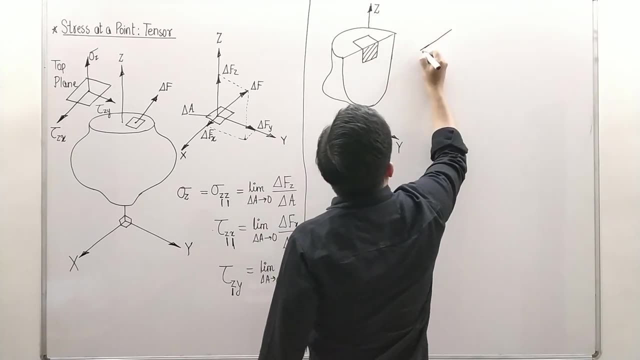 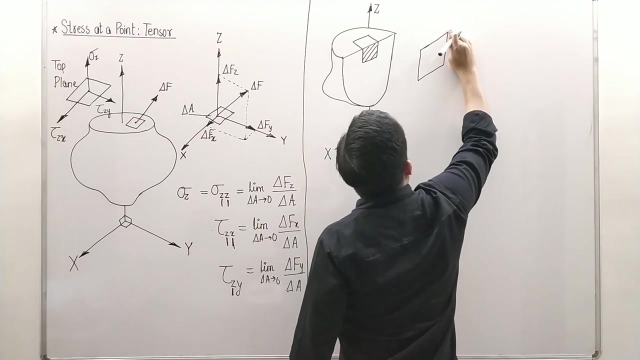 Let me try to make this plane over here, this plane. I'm talking about only this plane. Let me make it a, once again, a slightly bigger view. We'll try to see what's happening. Okay, As you can see, this plane is perpendicular to y axis. 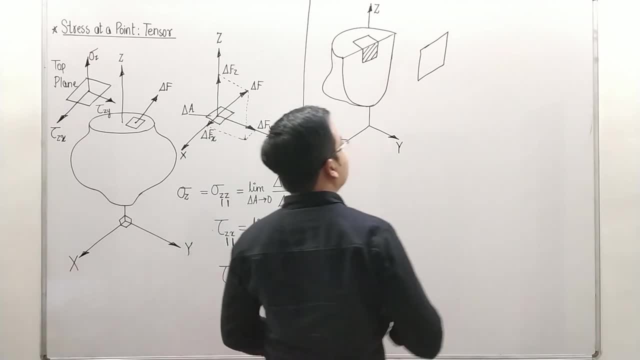 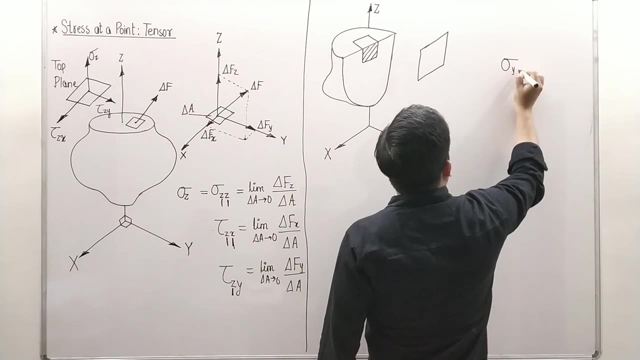 Okay, Now again, you'll be getting three components. What are they? Let me just tell you, You'll be getting sigma Sigma, what Y? Y? Let's see. You'll be getting tau. Yz, You'll be getting tau. 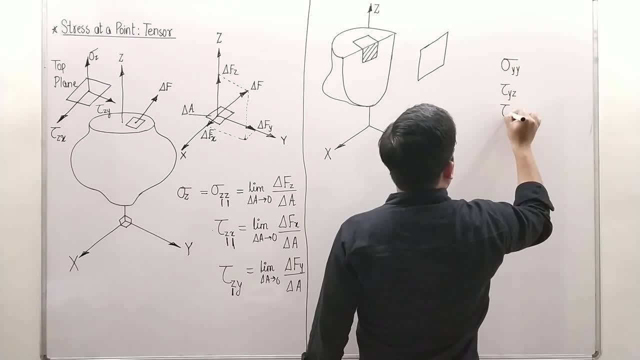 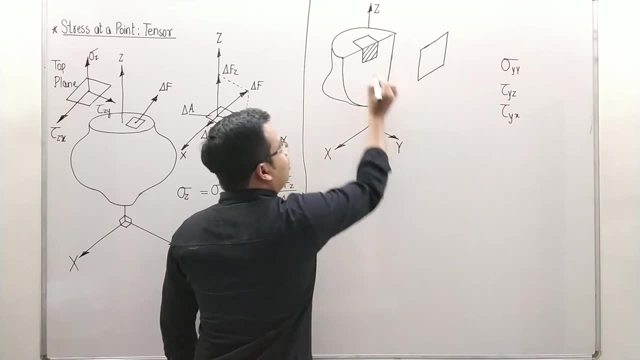 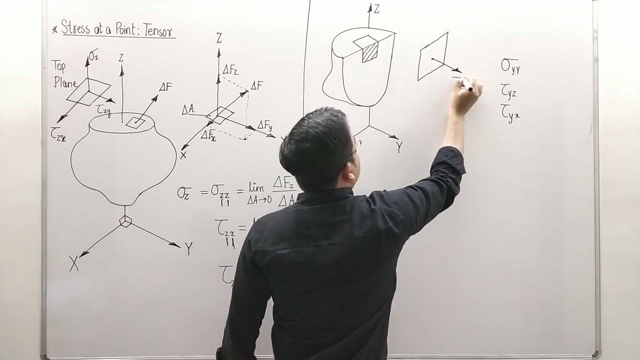 Z, Y, X. There you go. These are the three components which you'll be getting Now. this component component along this direction, this direction over here is perpendicular to the plane, So this has to be written as sigma yy. 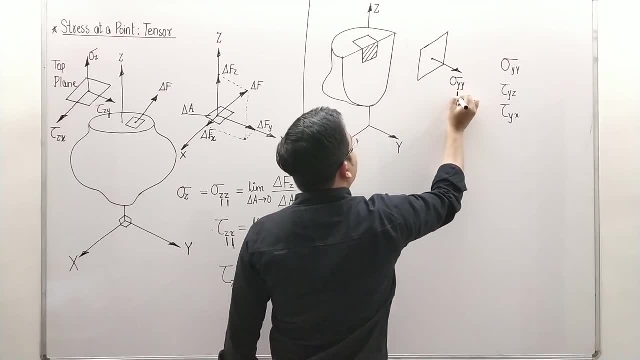 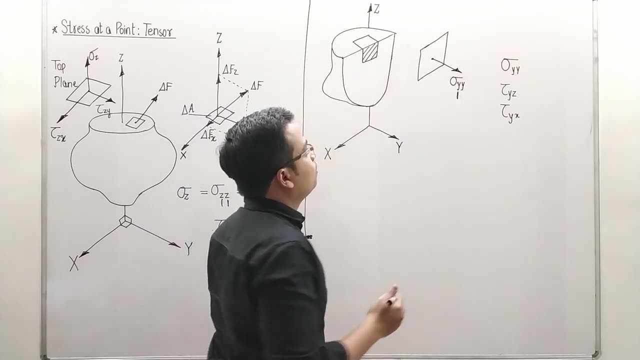 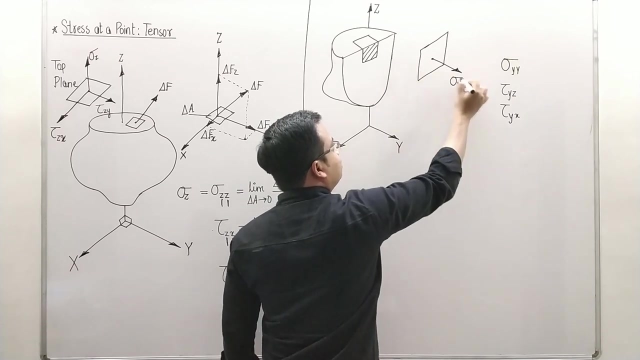 Y represents, since it is perpendicular to the. what should I call this? Stress on a plane perpendicular to y axis, along the y direction. Okay, So stress on a plane, on this plane which is perpendicular to y axis and in the direction. 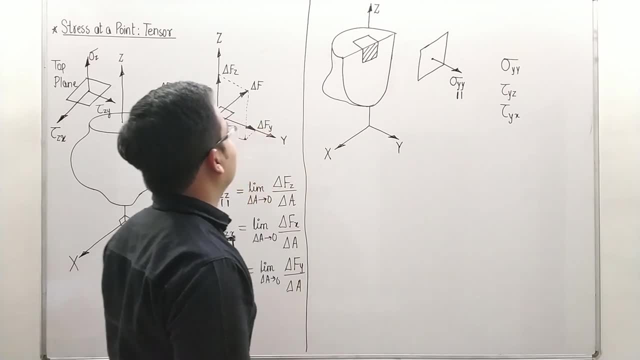 of y Done. Then there are going to be two more forces. Let me tell you, Those two forces are one in this direction and one in this direction. Okay, So these two forces are one in this direction and one in this direction. 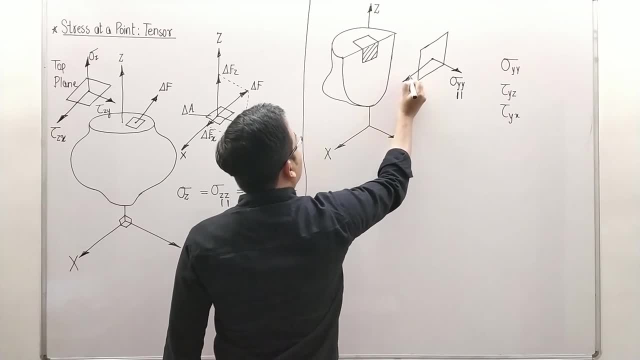 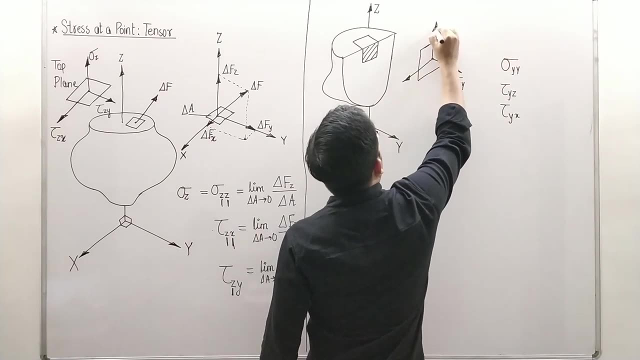 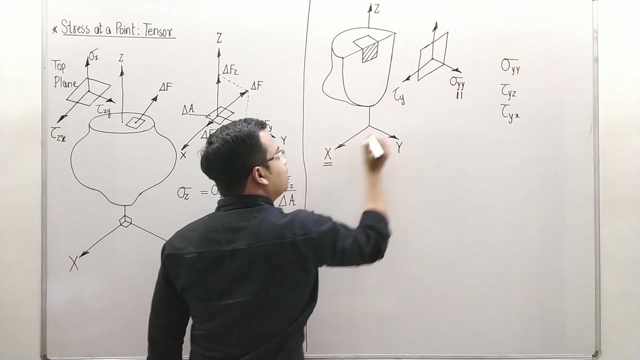 Okay, So these two forces are one along this direction and one along this direction. Okay, Here we go, While the other in the z direction, one along x direction and the other along z direction. So what about this? This is shear stress on a plane perpendicular to y axis, in the x direction, in the x direction. 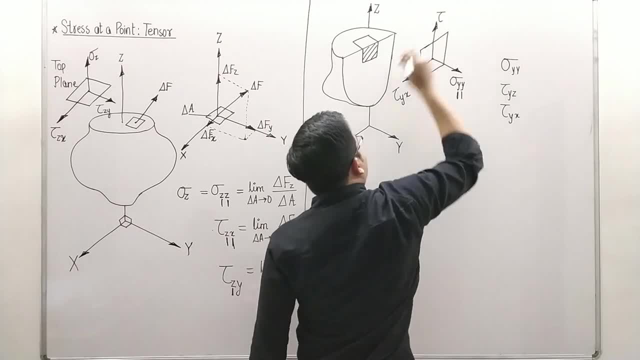 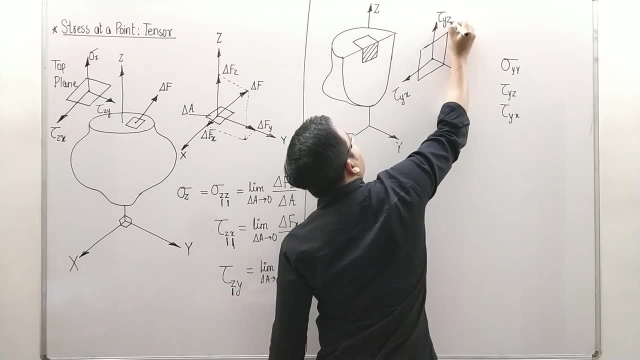 and this over here again is a shear stress- on a plane perpendicular to y axis. perpendicular to y axis, on this plane, and along which direction? and it is along the z direction. Okay, Z direction. So these are the three component of forces acting on this. let's say this over here: 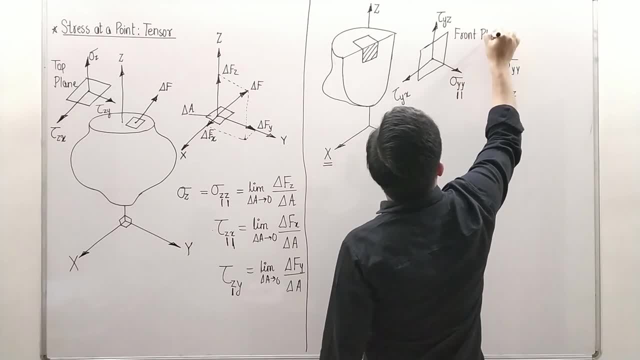 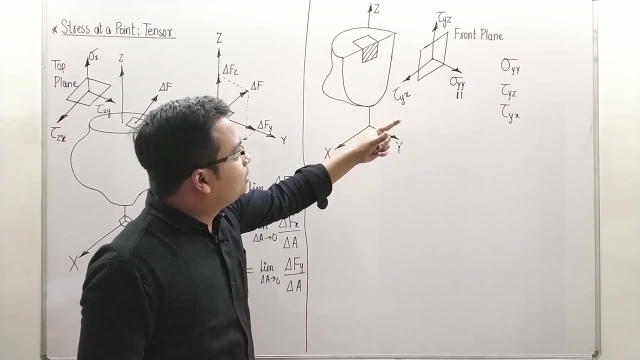 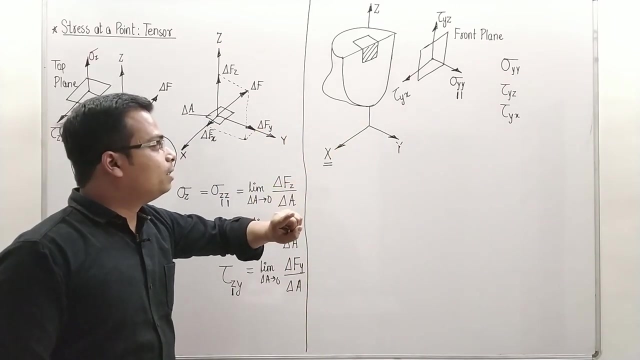 is a front plane. Okay, Don't go anywhere. I'm about to tell you what happens on a side plane also. So that's it. These are the forces acting. three more components. So we've got three over here, three over there, three plus three. how much Six? One more plane is left. Let me tell. 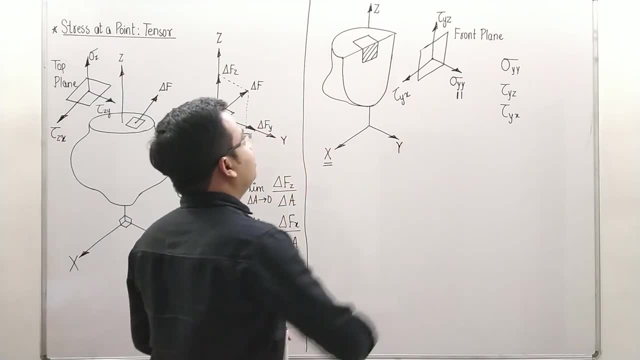 you what happens there? For that I need to cut it. cut it like this, Okay, With the help of a side plane. How would it look? First of all, let me think: Yeah, It will be something of this sort. 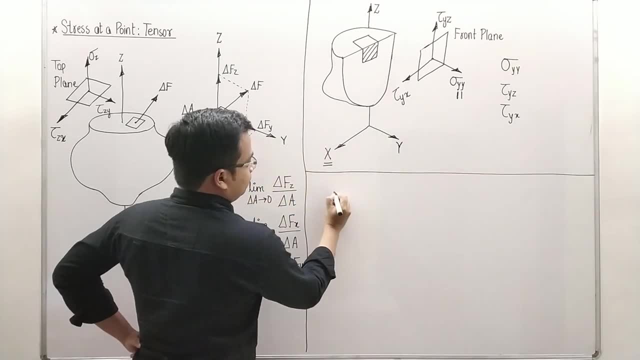 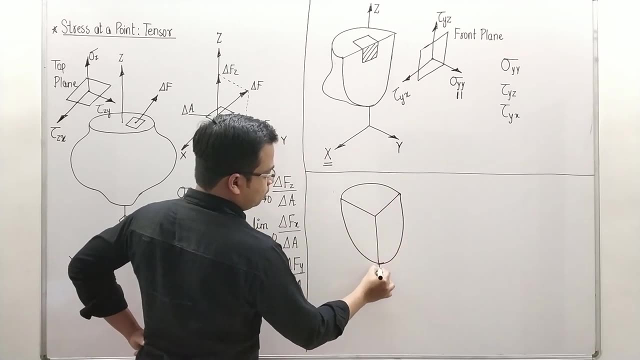 Let me have a division. Okay, So, so, so it's going to be something like this: Now again, we'll have two mutually perpendicular stresses Along these two direction and along this Z direction. So this is Z, for you That's Y, and 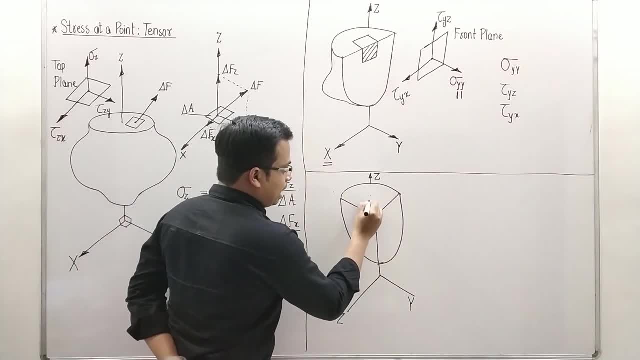 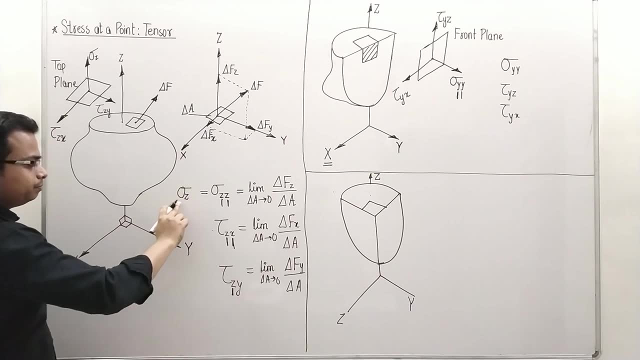 this over here is X. Now analysis for this plane. this, by the way, is the top plane. This over here is the top plane. The three stresses are acting: sigma, ZZ, sigma, not sigma, but tau ZX and tau ZY. 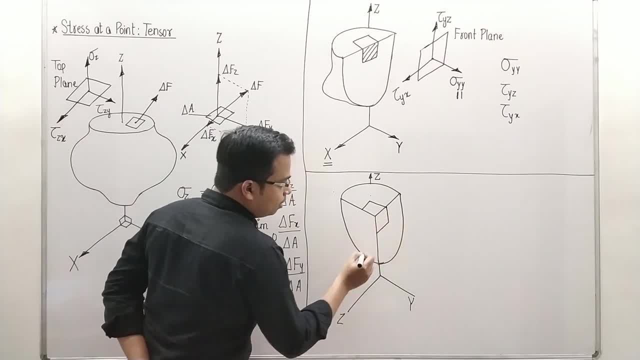 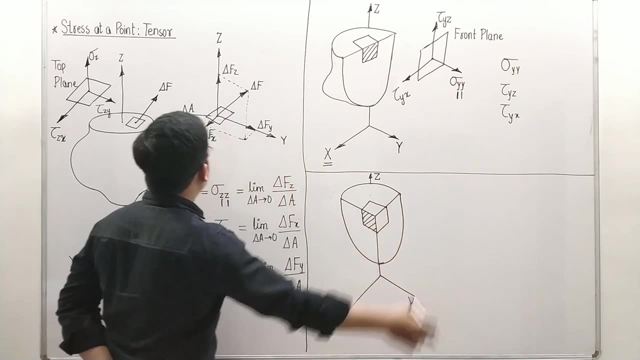 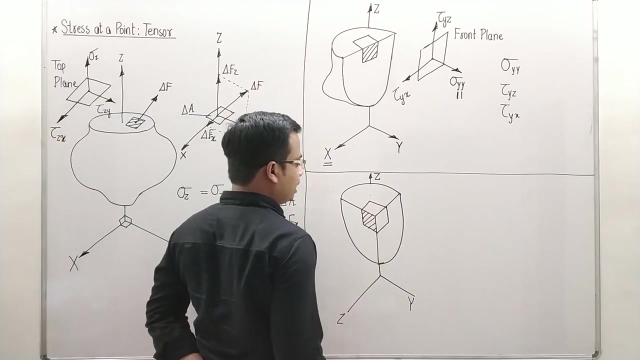 Analysis on this front plane also has been done, But the analysis on this side plane is yet to be done. This is something which I'll try to do over here. Okay, Let me just just highlight this. Okay, So what happens in this side plane? Let us try to work it out together. So it's: it's something like: 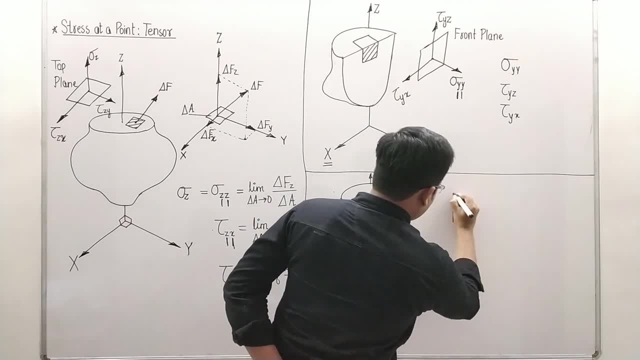 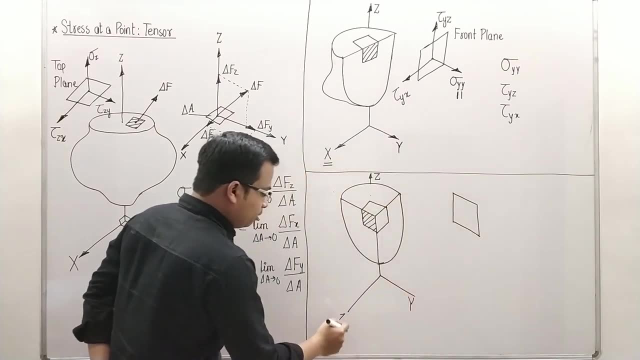 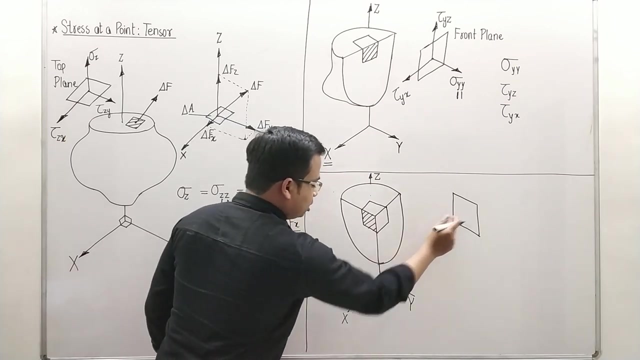 this What's happening inside this side plane. Okay, So this plane is perpendicular to what? Perpendicular to the? this is not Z, this is X. Okay, So this plane is perpendicular to the X axis, So one component of stress will be along. 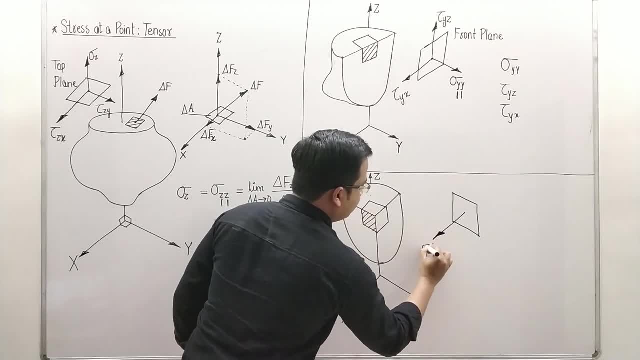 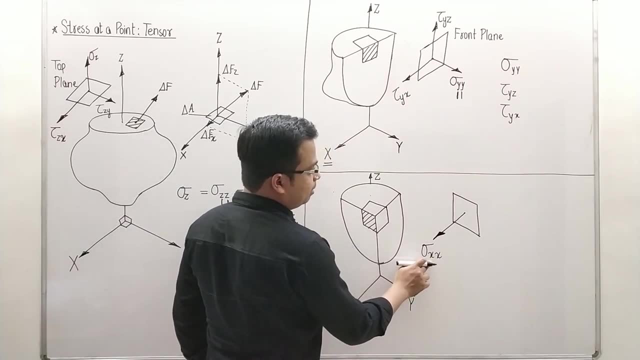 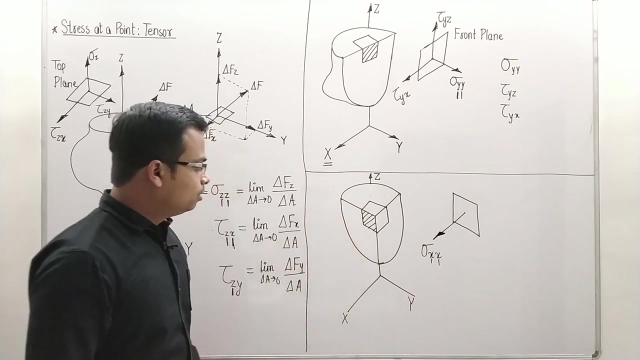 this direction And this is going to be what you call sigma X, simply sigma X. You can also write it as sigma XX. So normal stress on a plane perpendicular to X axis. done in the direction of X, in the direction of X, Done Okay. Now there are going to be two more stresses, and both of them. 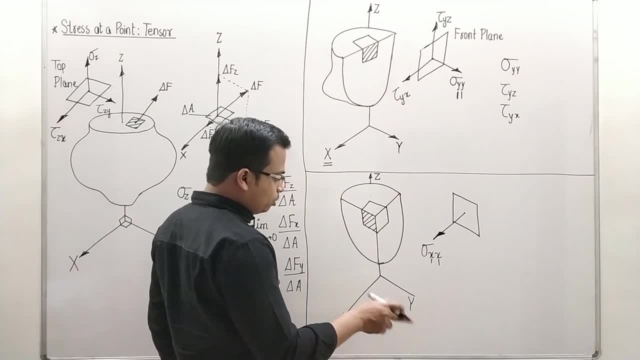 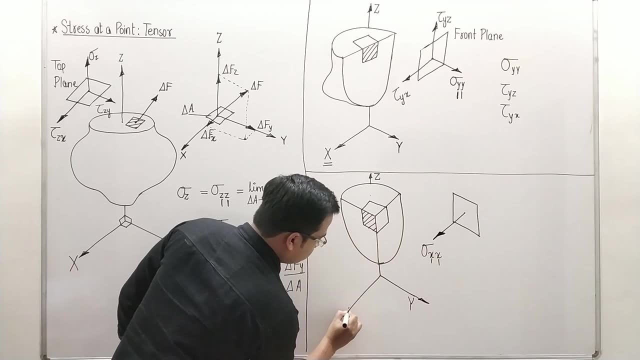 are shear And if you watch carefully, one is along one, one is going to be along the Y direction, One is going to be along the Z direction. So the Y direction is over here, Let me make this, and one along the Z direction. So one stress is going to. 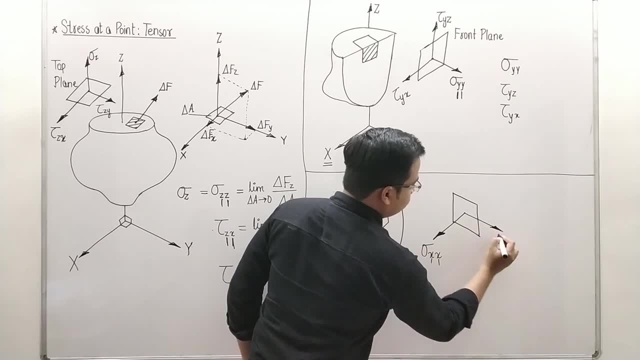 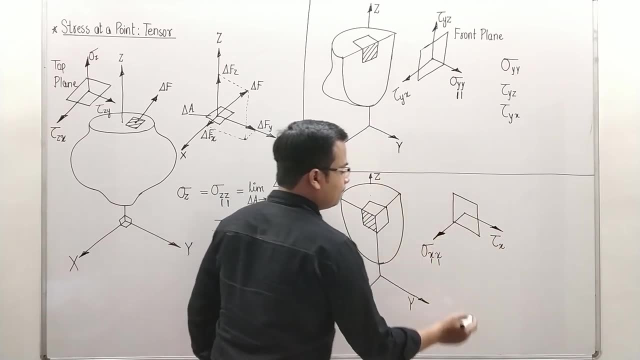 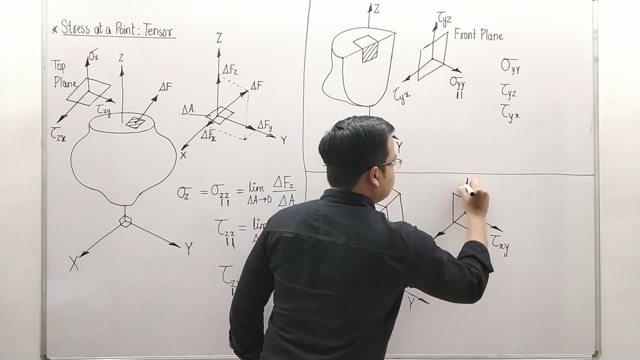 be along this direction. So this is going to be tau. Sheer stress on a plane perpendicular to X axis. perpendicular to X axis. We have this plane in the direction of, in the direction of Y Done One more left. You have this shear stress on a plane. 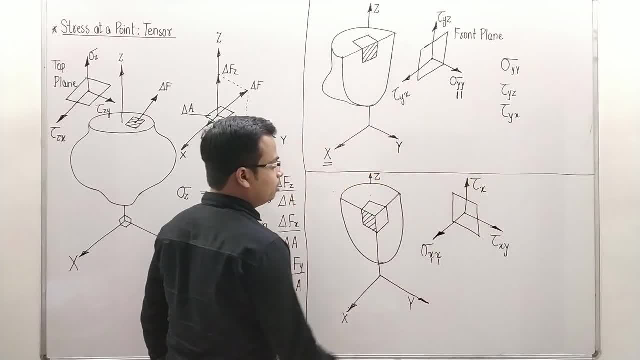 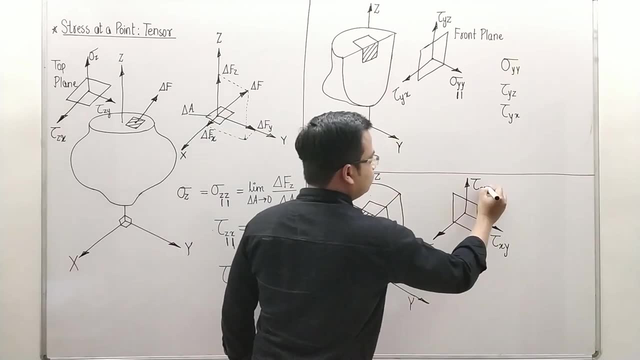 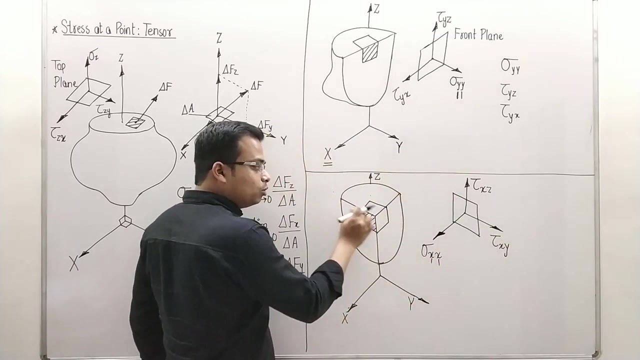 perpendicular to the X axis. Okay, Perpendicular to this X axis, You've got. perpendicular to X axis, You've got this plane, this plane I'm talking about, and in the direction of Z. Now you know, there are three components of stress onto this side plane also. Their names are sigma. 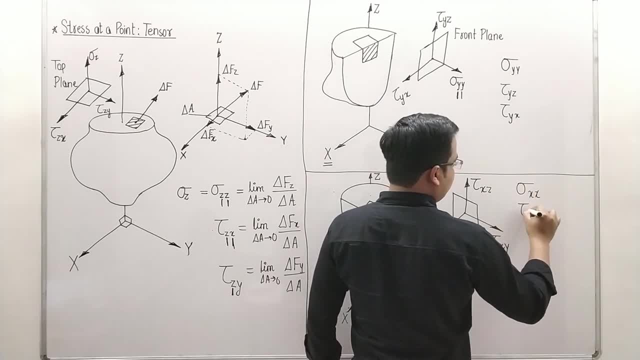 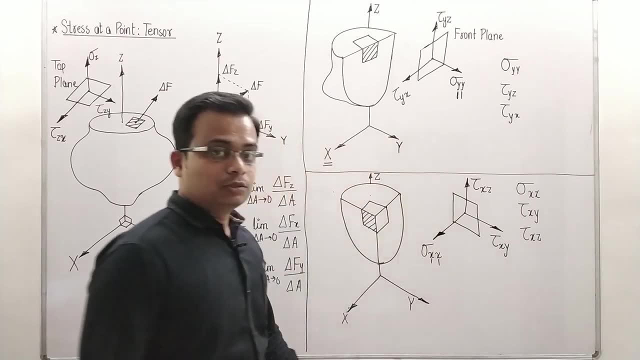 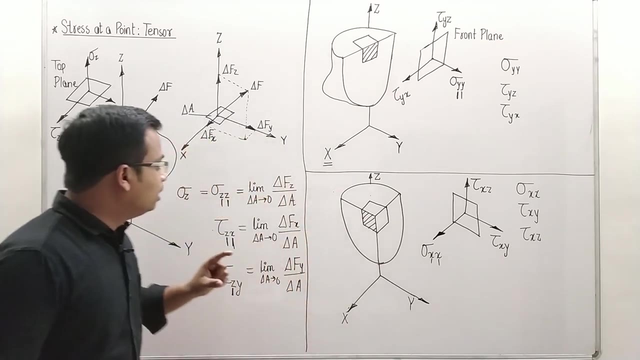 sigma what Sigma XX? Then there is tau XY, Then there is tau XZ. So this was all about stress acting at a particular element, And this element is extremely small. Why is it small? Because everywhere we have done this delta eight. 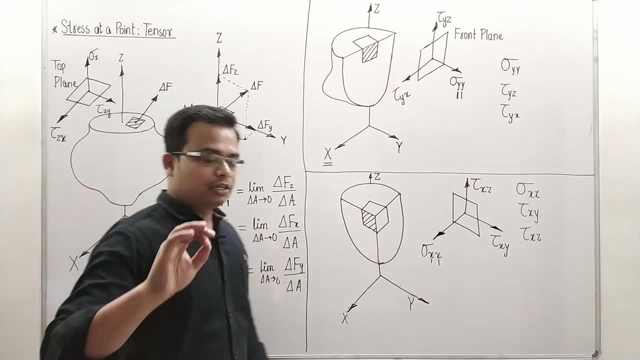 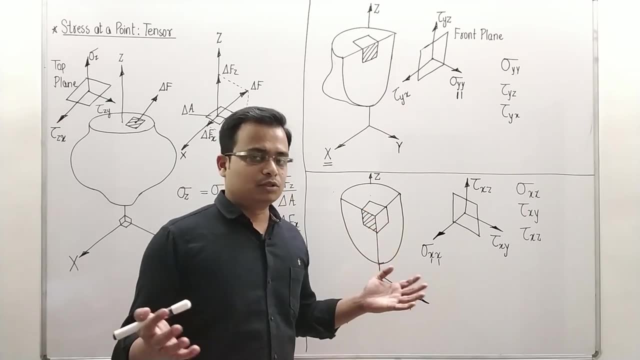 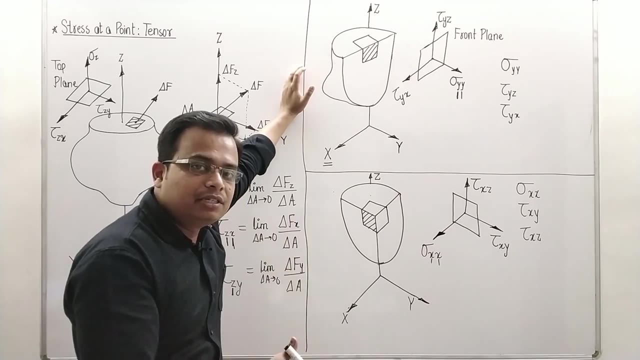 into zero, delta eight into zero. So these are all the values for stress at any point inside a rigid body, when it is, say, when it is pulled or pushed by external forces. Now I'll let you know how a stress matrix is formed, how all these nine components are written in the matrix form. 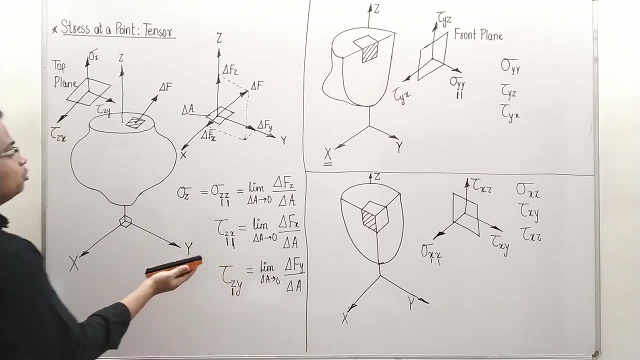 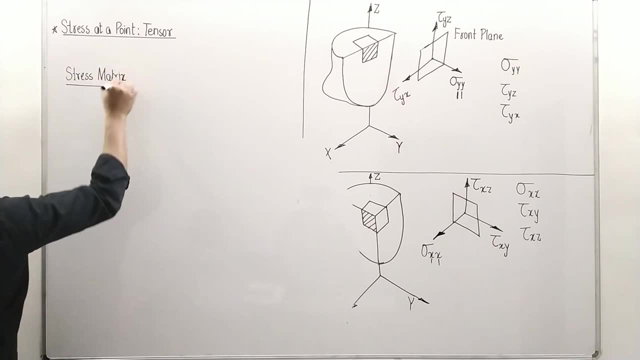 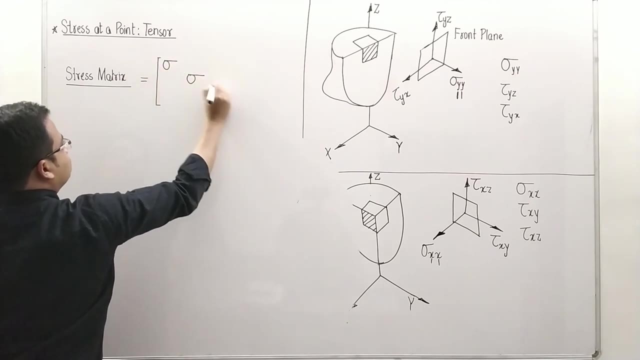 So let's see that. Why wait? Okay, So I've got to rub all of this Stress matrix. So it's like this: First of all, you should try to remember: Just write down sigma, sigma and sigma. along the diagonals X, Y and Z: Tau, tau, tau everywhere. The remaining spots: Tau everywhere. 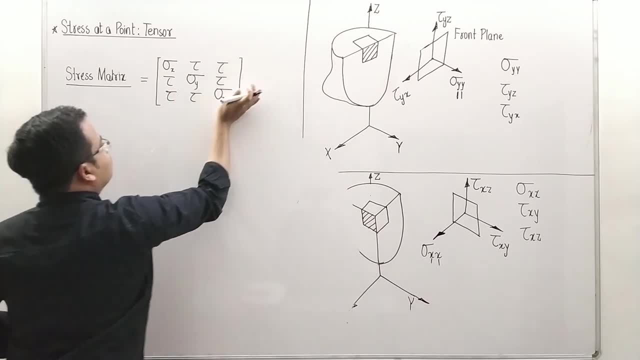 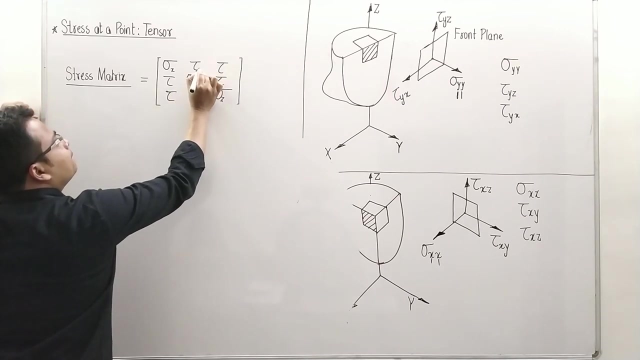 Okay, And let me just finish this up. So for normal stress, I'm just writing X. I'm not writing XX or YY or ZZ Right On a plane perpendicular to X axis. So just write tau, XY, Shear stress on. 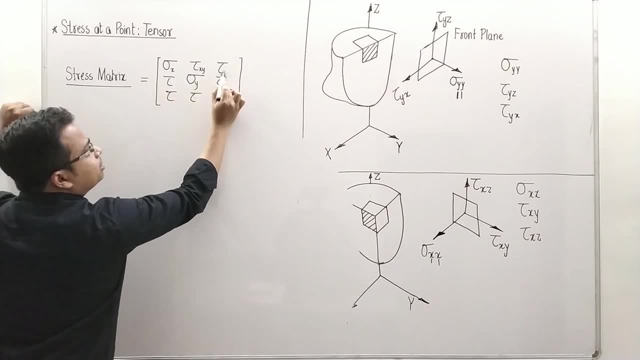 a plane perpendicular to X axis in the Y direction. Shear stress on a plane perpendicular to X axis in the Z direction. Shear stress on a plane perpendicular to X axis in the Z direction. Shear stress on a plane perpendicular to Y axis in the Z direction. Shear stress on a plane. 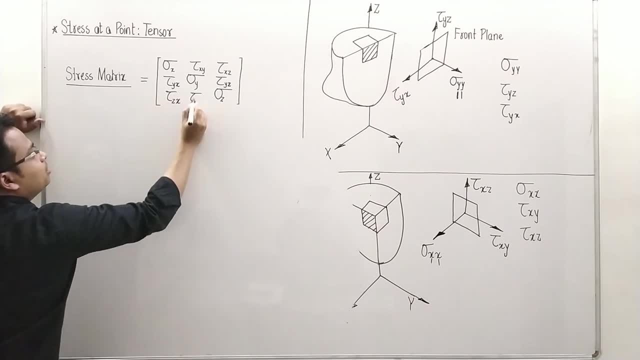 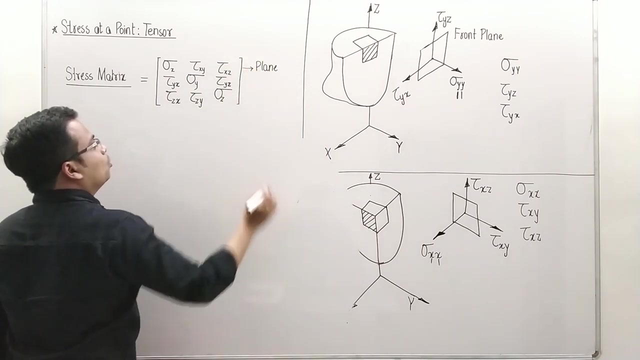 perpendicular to Z axis in the X direction. Shear stress on a plane perpendicular to Z axis in the Y direction. So what does a row represent? Row represents the plane. Okay, So which plane is this? This plane is perpendicular to. I need to make more space. 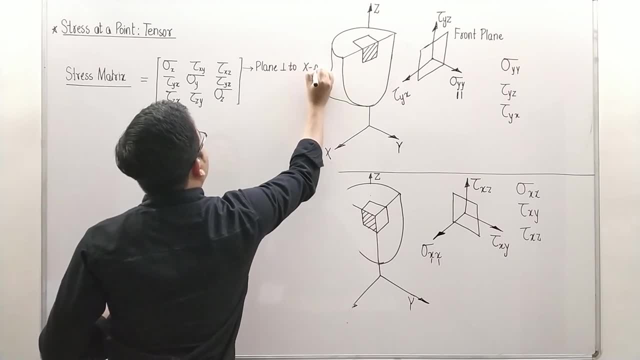 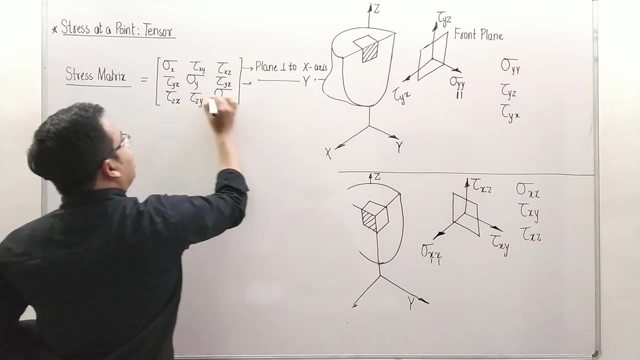 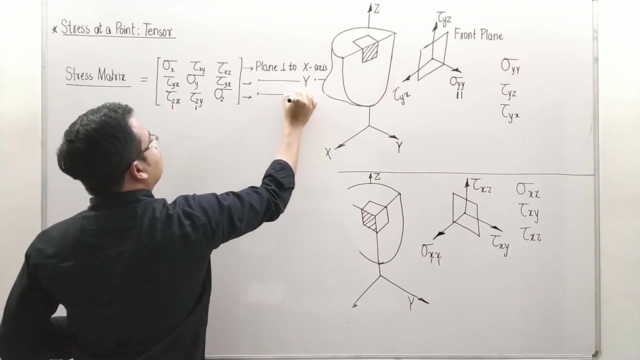 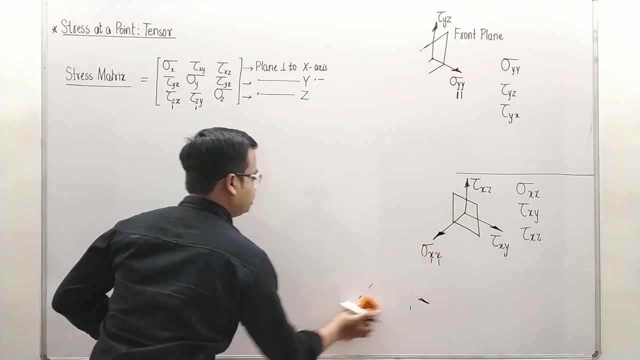 This plane is perpendicular to X axis. What about this plane? Here the plane is perpendicular to Y axis. And this third row: here we have a plane which is perpendicular to Z axis. Done So, this is how representation is being done. Now, how do you read the columns? So, 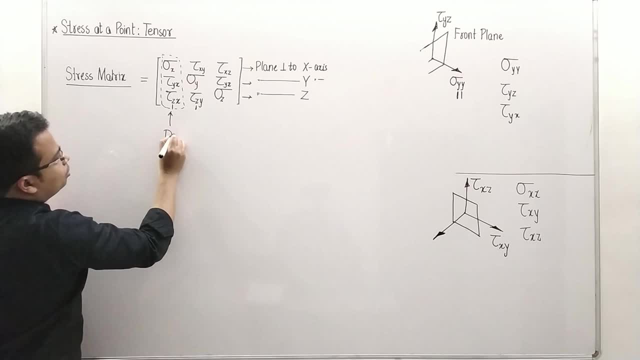 when you talk about column, all of them show direction. Now, this over here shows the direction along X, This shows the direction along Y And this over here shows the direction along Z axis. Done, It's that easy. Subtitles by Prof Arun Mittal. 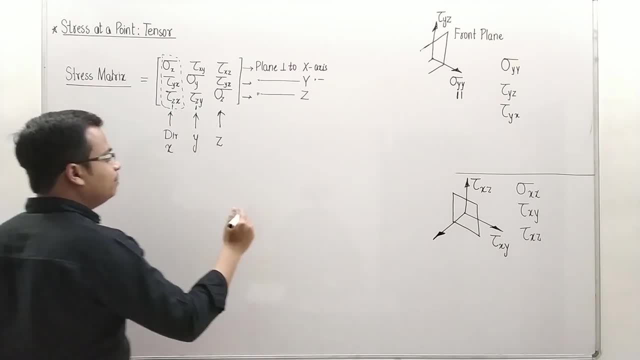 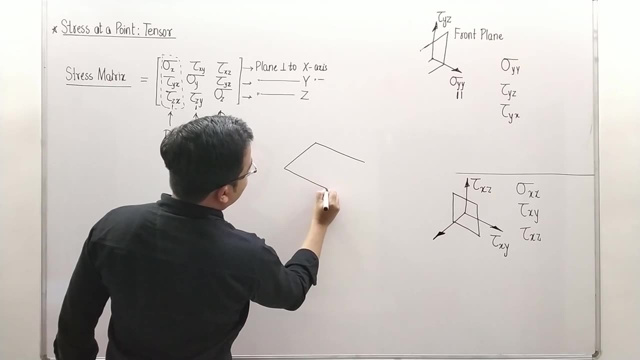 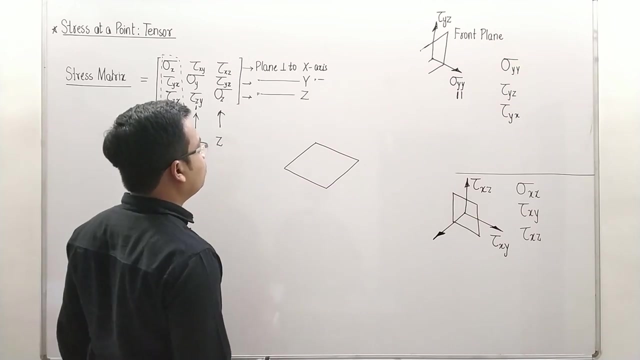 Subtitles by Prof Arun Mittal. Subtitles by Prof Arun Mittal make a stress element. how can that be achieved? Well, it's going to be something like this. Let me make it. Yeah, This right over here is the top plane. Okay, So when I talk about a top plane, 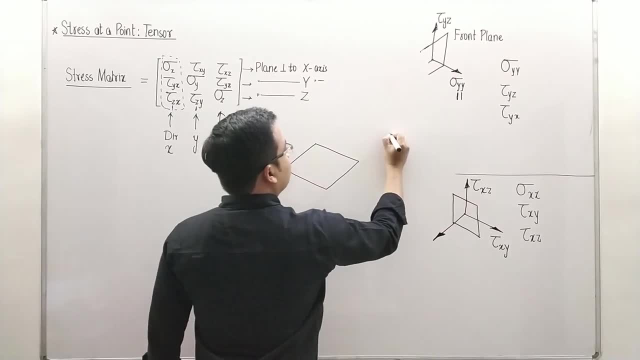 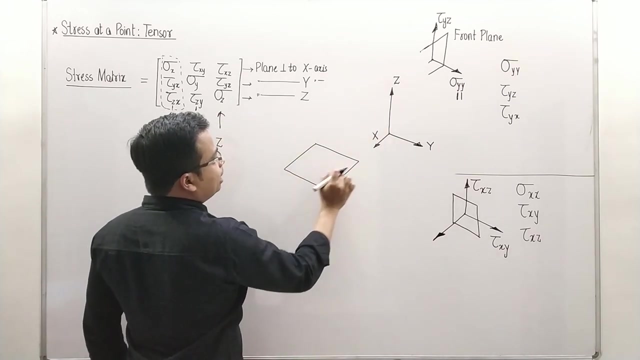 there are three stresses acting on it. One is, first of all, let me make this coordinate axis. This, by the way, is the z-axis, This is your y and this is x. Okay, So when we are talking about, 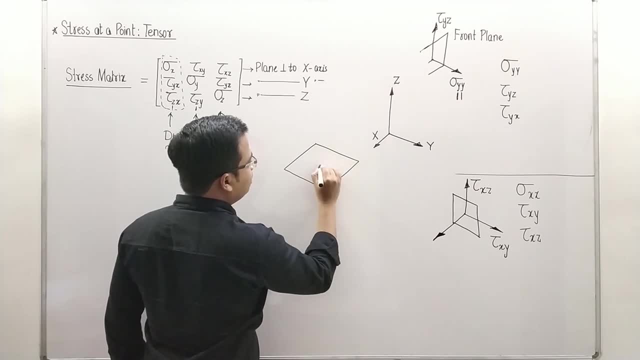 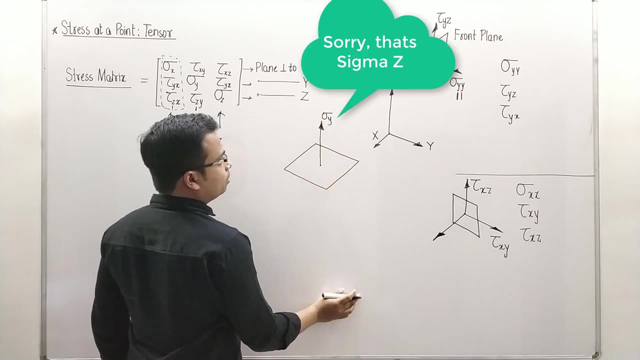 the top plane there are three stresses acting on it. Right at the center- let me try to make this Here- we had sigma y Okay. Then, along this y direction, we had a shear stress Here. this was the direction of shear stress Tau. 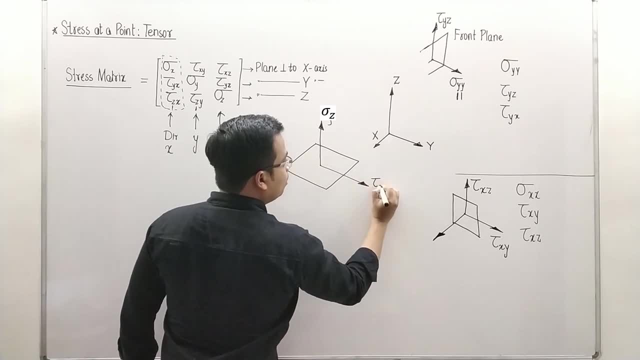 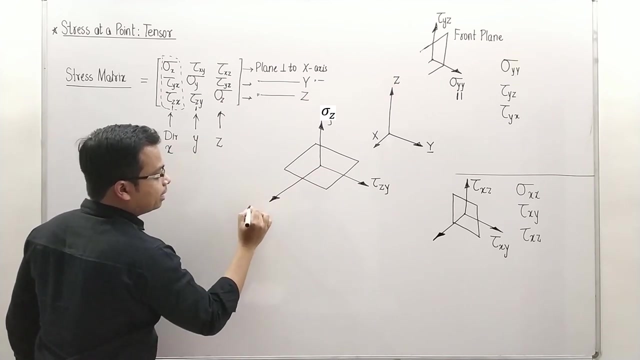 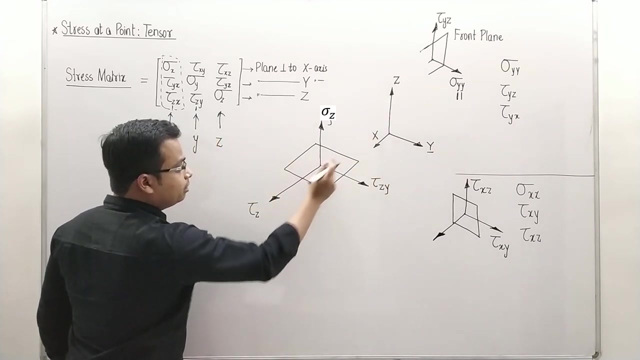 tau, this has got to be tau- on a plane perpendicular to z-axis, on a plane perpendicular to z-axis in the direction of y. Then we had one more. This is again shear stress on a plane perpendicular to z-axis. You got this plane on plane perpendicular to z-axis, in the direction of x. Okay Now. 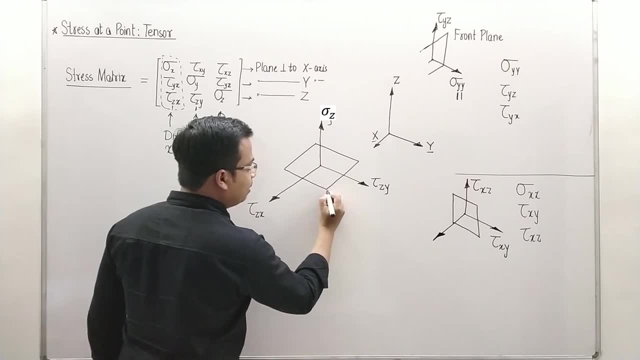 after this, we we did half section with the help of a front plane And we got this. Let me make this. Takes time to make these joints. Now what happens? Again? there are three stresses acting One over here, So instead what I will try to do is: 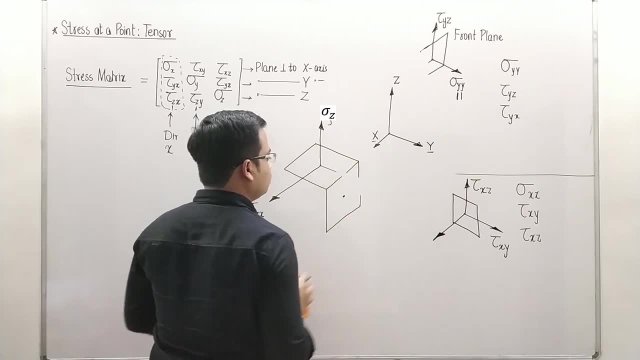 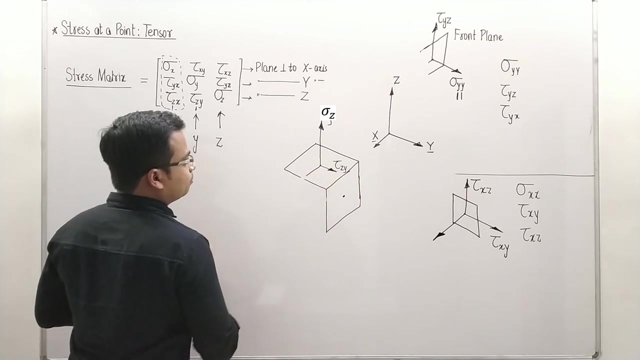 let me shorten this, Okay. So this is what this is: tau tau, what tau z on a direction perpendicular to z-axis, in the direction of y, And we- let me shorten this also- Why do we need so longer arrows? Okay, What is this? It is tau z on a plane perpendicular to z in the direction of x Done. So these are the three stress driving forces that are acting as part of there. So this is what I will shortly get into after. Let me shorten this also. So this is the lieutenant's state disrespect about that and a lot of of what he's saying. So let me shorten this: לה Head perpendicular ñ manager, whose home deduct. What are his expressions? We can't alloccup знаешь him to just talk about it. Okay, What is this? This is tau z on a plane perpendicular to z in the direction of x Done. 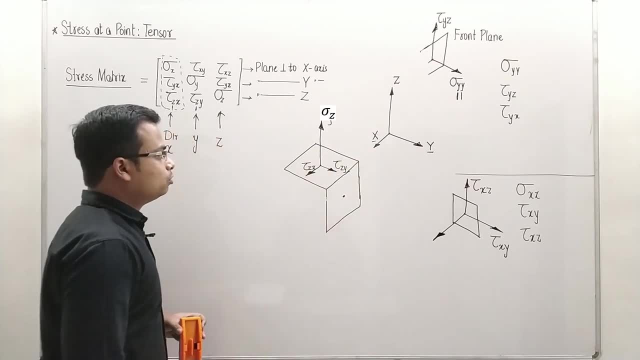 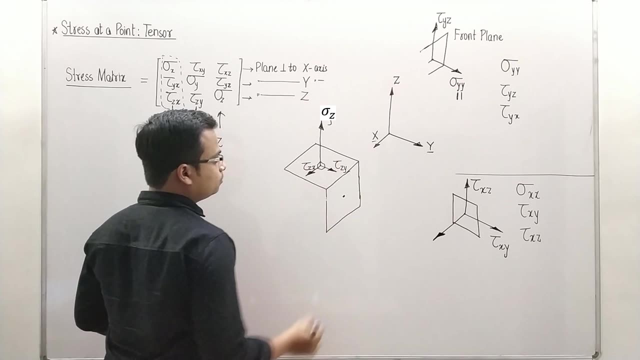 tauесd on a plane perpendicular to z in the direction of z Done, is acting Okay, And all of them are. by the way, they are also mutually perpendicular. Okay, Now let us talk about this first. Well, perpendicular to this plane, we have got a. 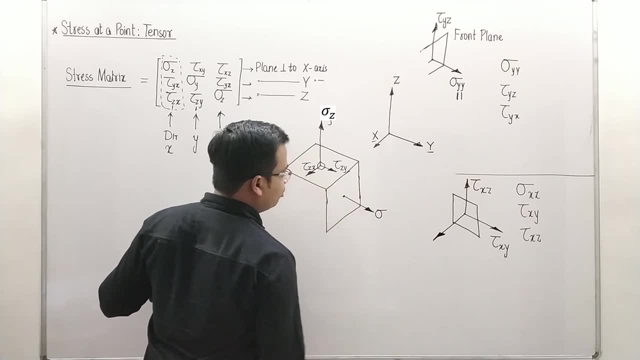 stress of this soil. Since it is perpendicular, it has to be denoted by sigma Perpendicular. to which axis Y, axis subscript 1.. Then, in the direction of what? In the direction of y. So either you can write this, also better try to avoid it. Okay, Then there are two. 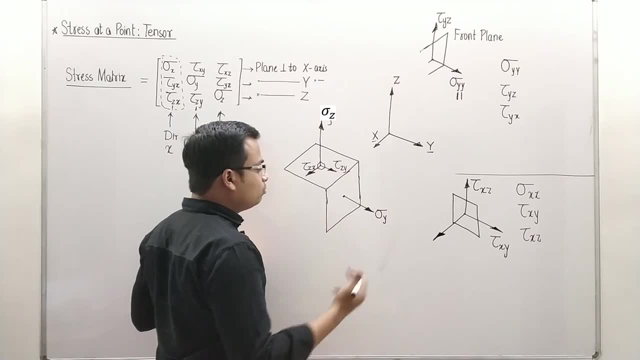 more stresses acting. One is shear. Well, both of them are shear, in fact. Okay, One along this direction. What is this? This is tau, where, on a plane perpendicular to y. in which direction X. Then there is one more here, Okay, On a plane perpendicular to y. 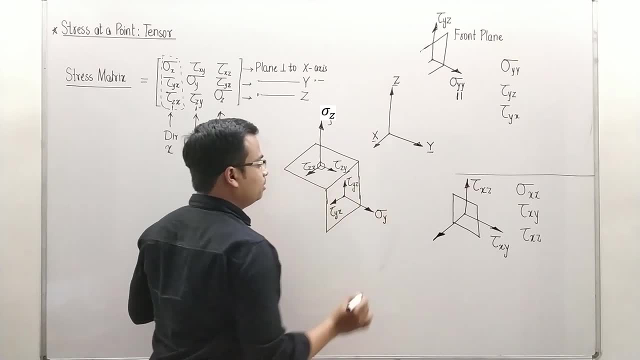 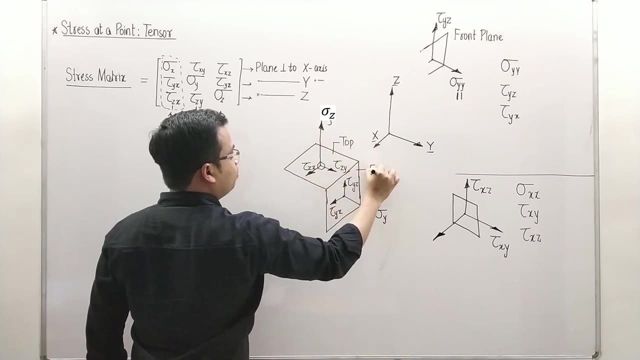 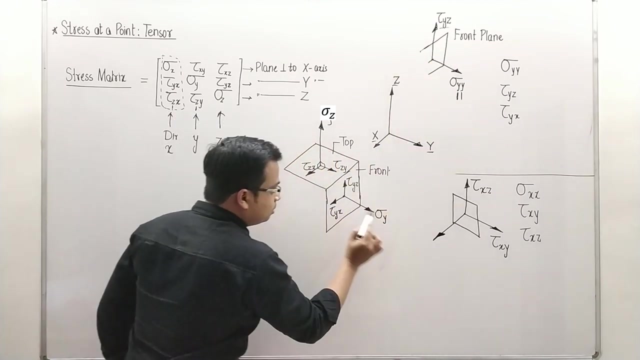 axis. in which direction? In the z direction. That is it. So this, by the way, is the top plane. This, by the way, is the front plane. Okay, I drew the front plane over here. You can clearly see tau y z upward, sigma y y, sigma y y. and there was one more over here, Okay, 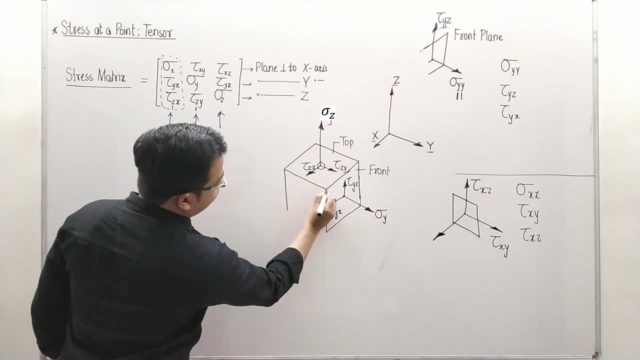 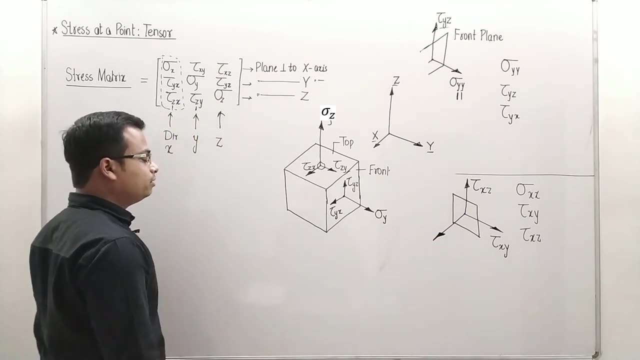 And there was one more plane which you saw. This is the side plane, Right. How to make this? This is also fairly simple. Now let me mark the midpoint. So what happens is now perpendicular to this plane. first of all, you got a stress. 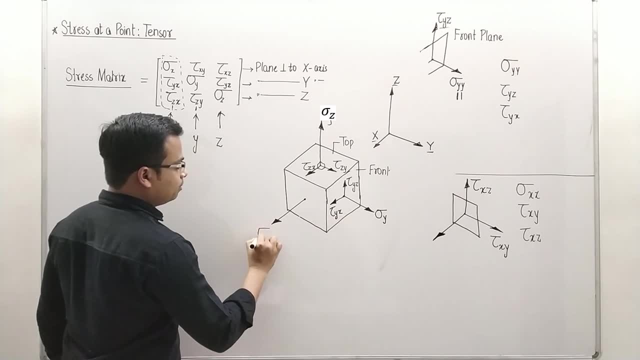 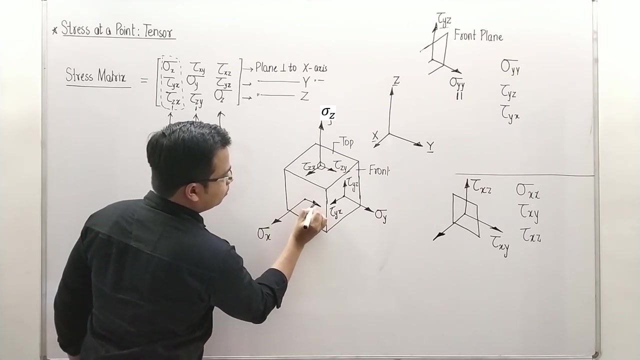 in this direction. Okay, So this is on a plane perpendicular to x axis, Done In the direction x also. Okay, Now there are two things left, y and z. So you are going to have one shear stress in this direction, and by now I am pretty much sure that you must.